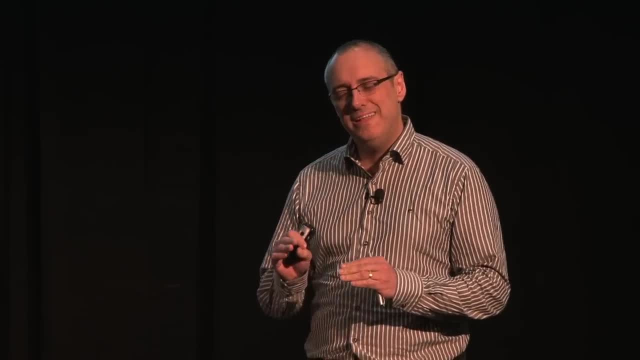 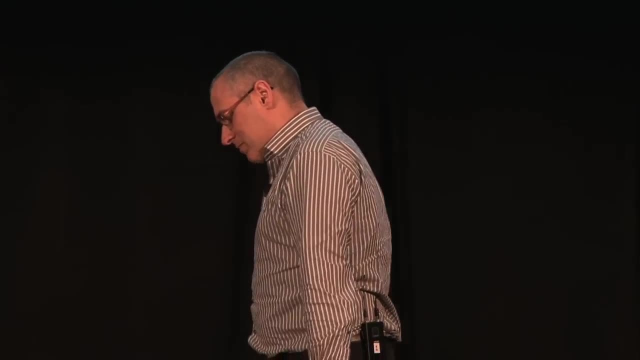 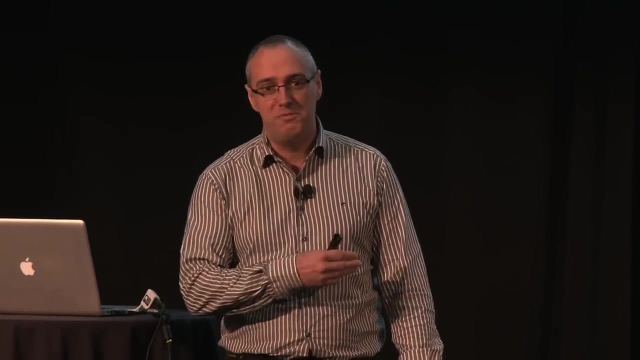 the talk of Randy. I'll be a little bit over some of the things he said. It's inevitable somehow. But I'm from the CMS part. He's from the Atlas part, I'm from the CMS part. Anyway, we are the same community, So you will be hearing most of the same stuff at the beginning. 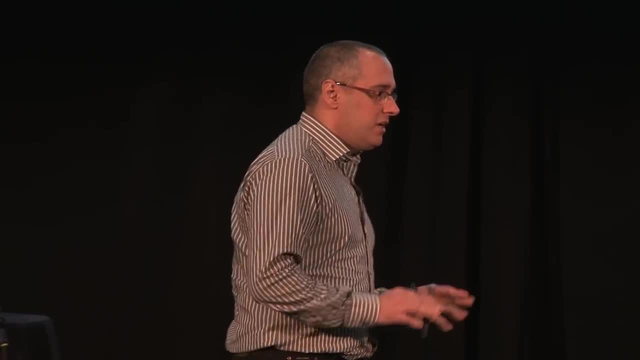 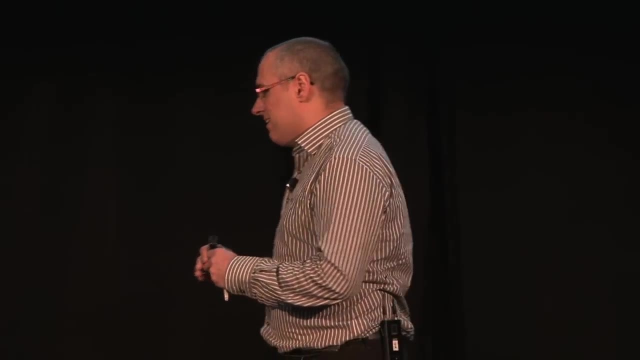 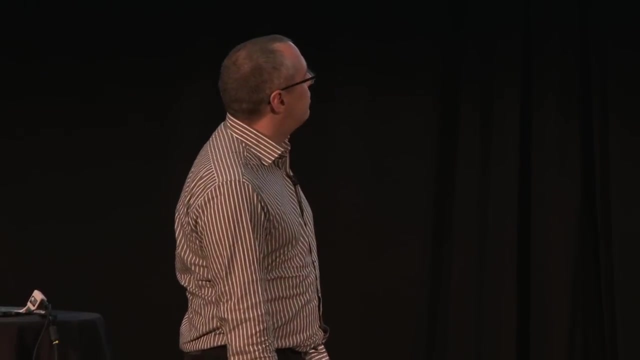 from his talk And I will zero in into what we did actually in this deployment of Open Stack as a rather not common way, because for us it's an overlay layer, as you will see, And this work we did in CMS, I did it basically with Wojciech, which is a marvelous 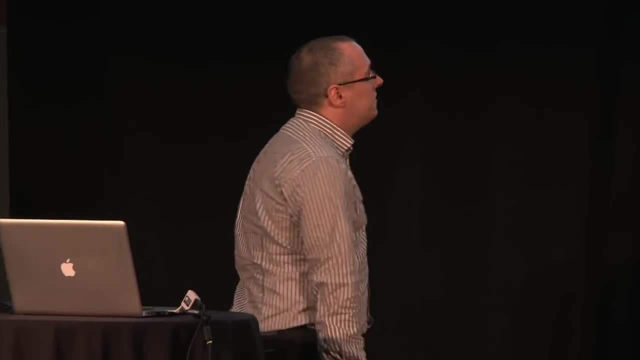 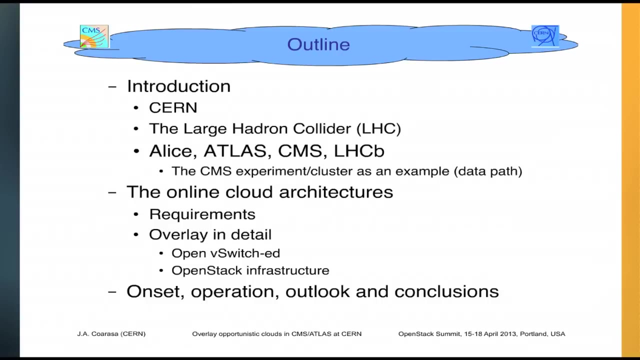 student. So let me start. This is basically the outline of the talk. I will introduce CERN, introduce what we do there, introduce what the experiments do there, And then I will Explain a little bit more in detail. Why do we have the computers we have? What do? 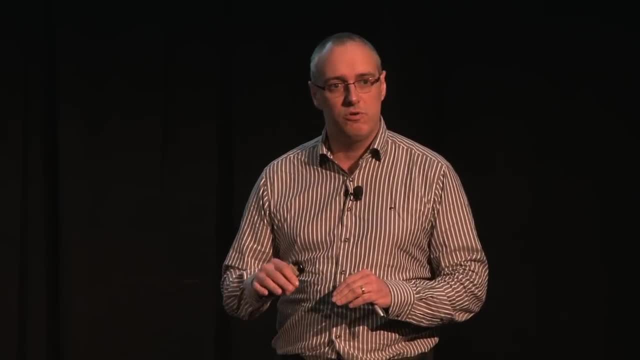 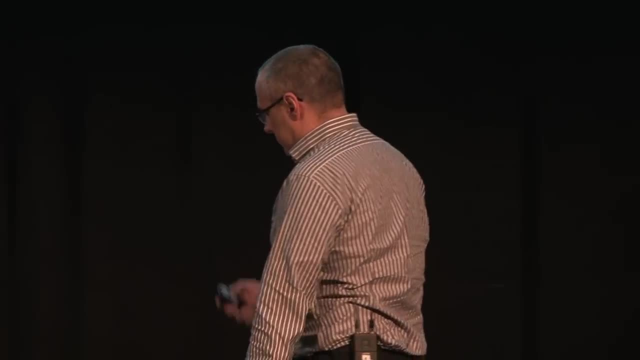 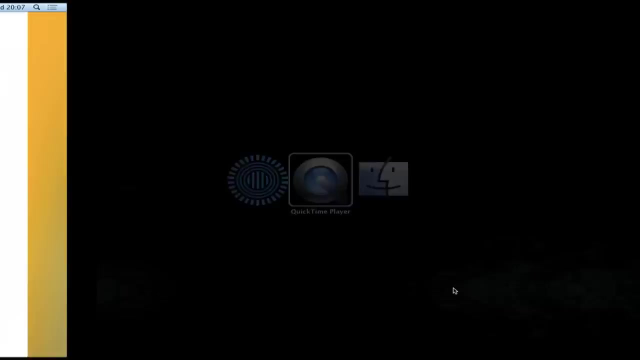 we do with them. And then, what did we do? to deploy Open Stack on top of it as an overlay layer And allow us to do more things that we couldn't do before, But actually to introduce CERN. what I will do, instead of doing something myself, is: 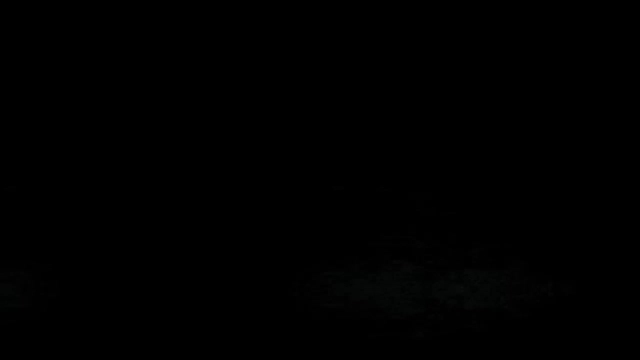 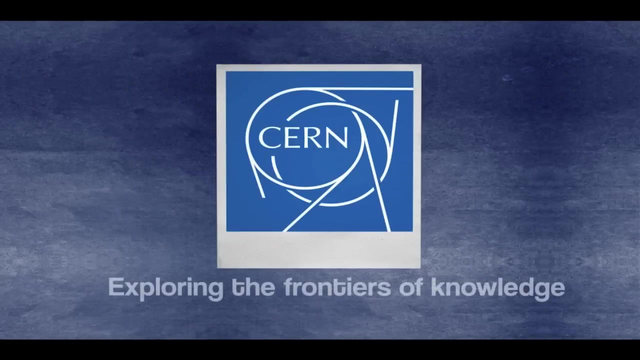 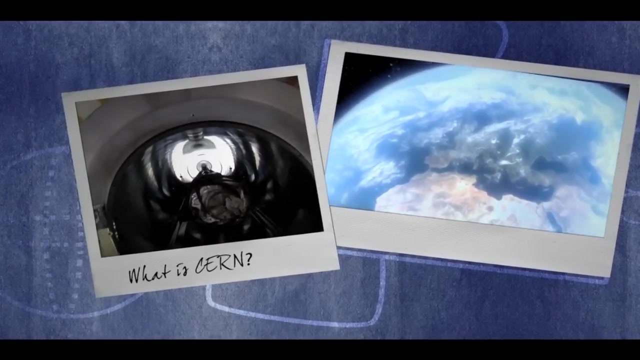 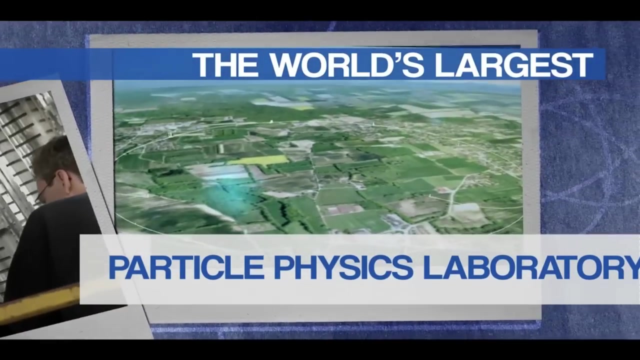 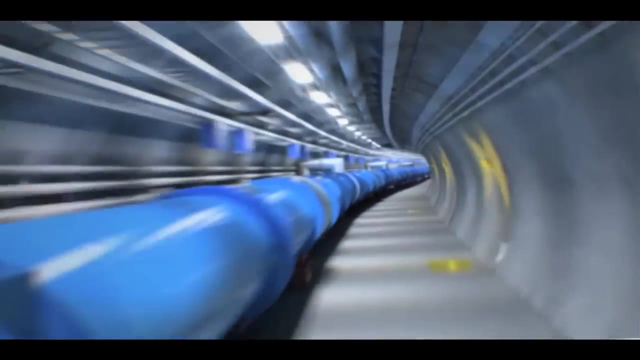 just run a video. I hope you enjoy it- from outreach people, Okay, So let me just run the video. I think we are running. 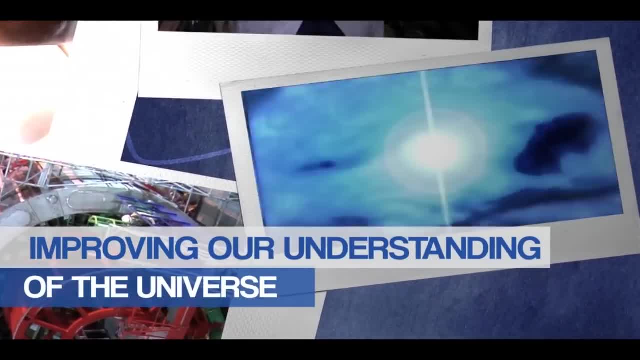 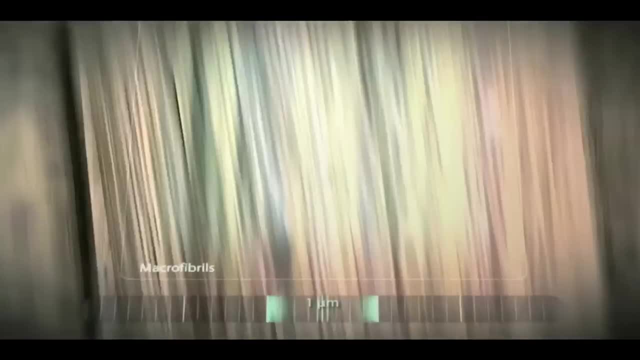 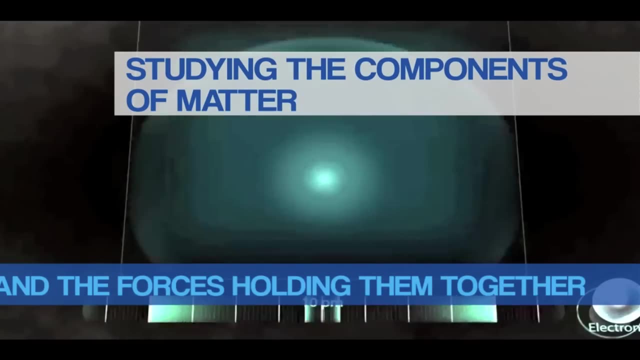 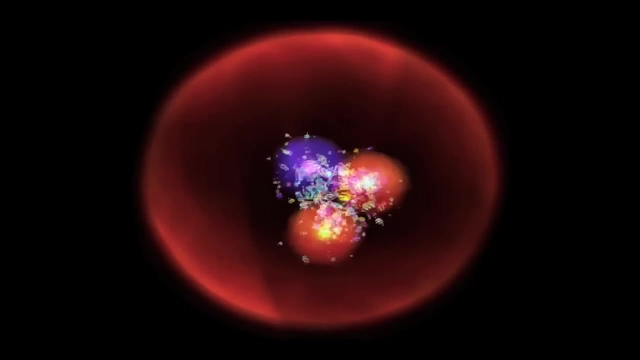 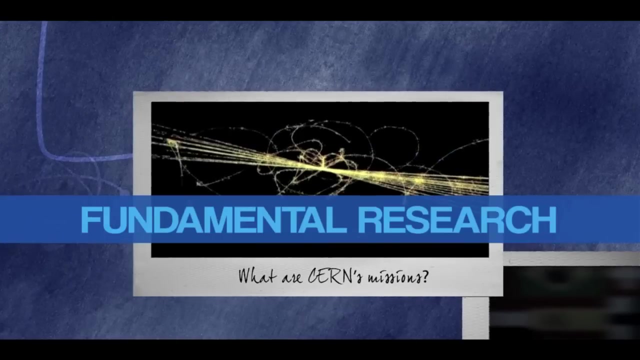 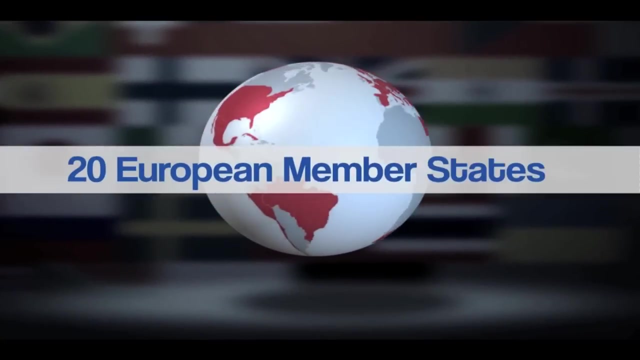 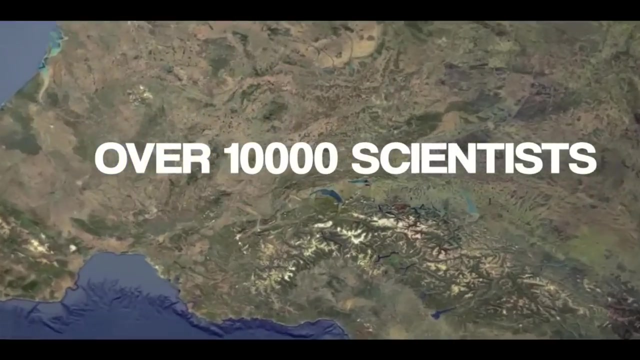 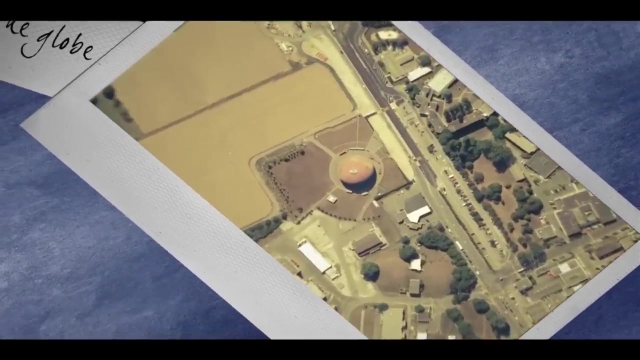 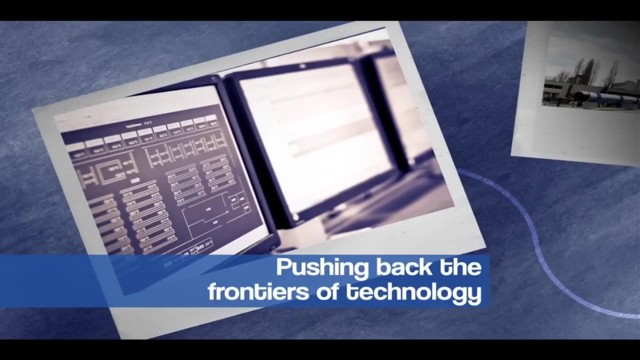 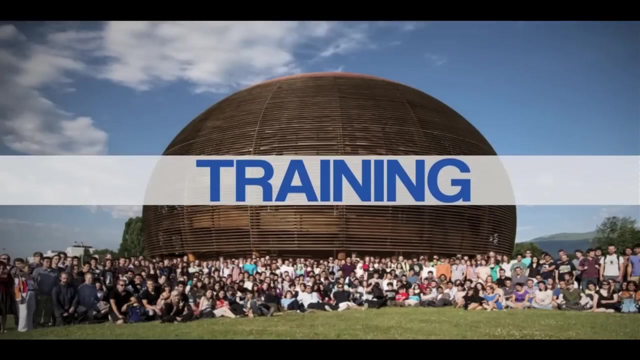 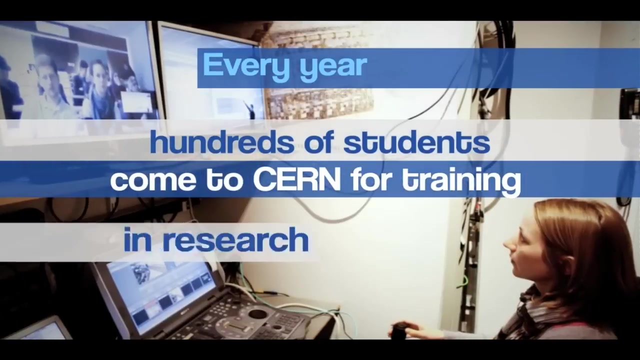 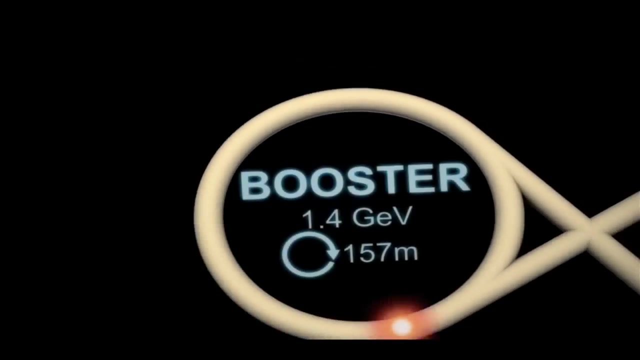 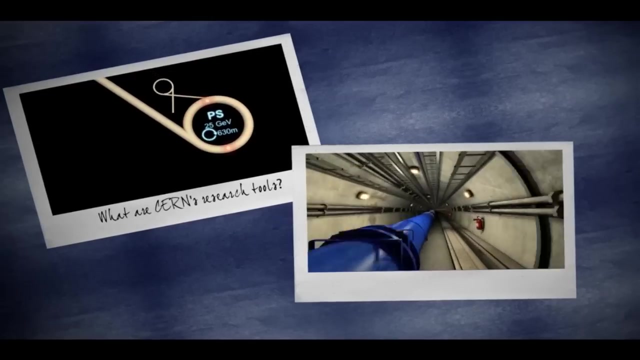 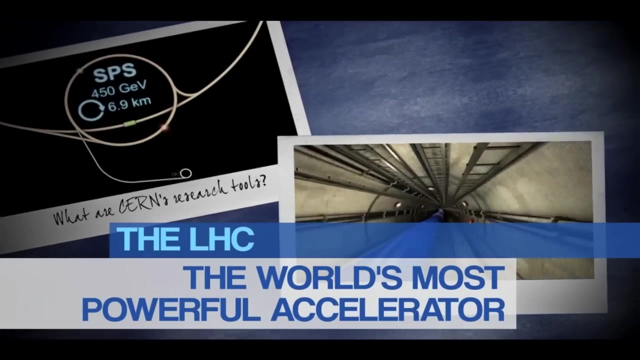 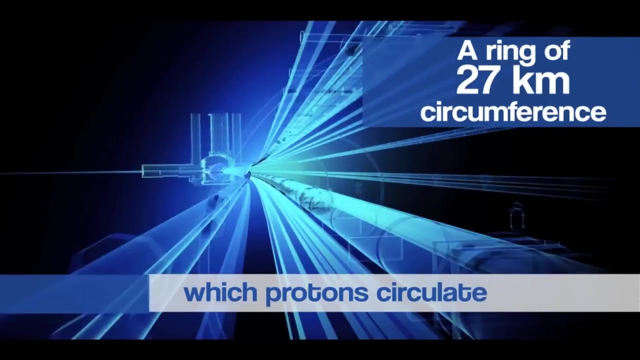 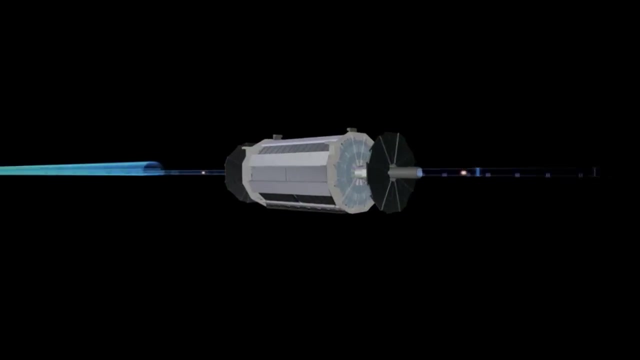 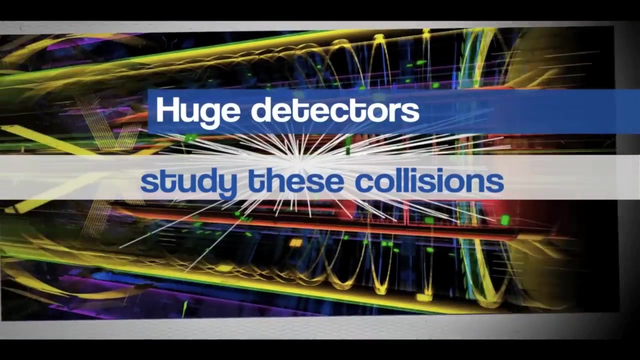 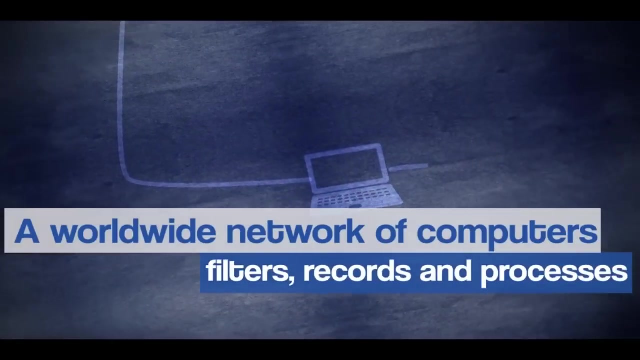 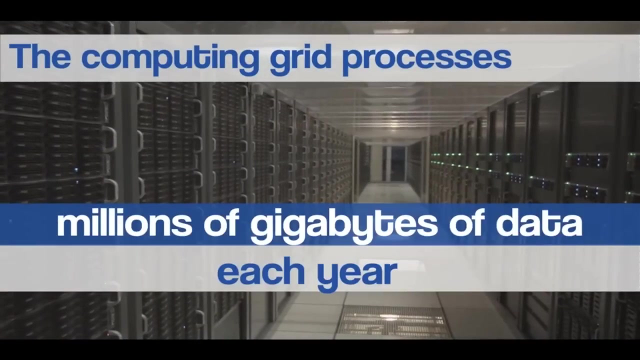 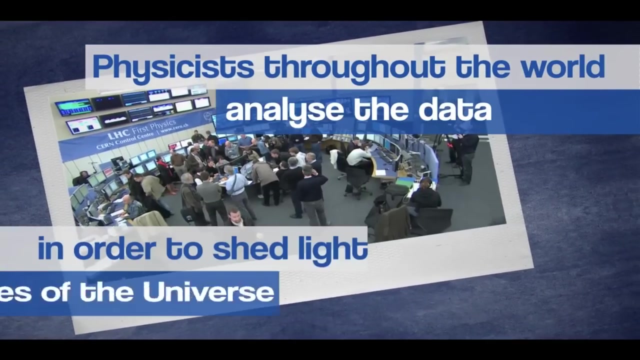 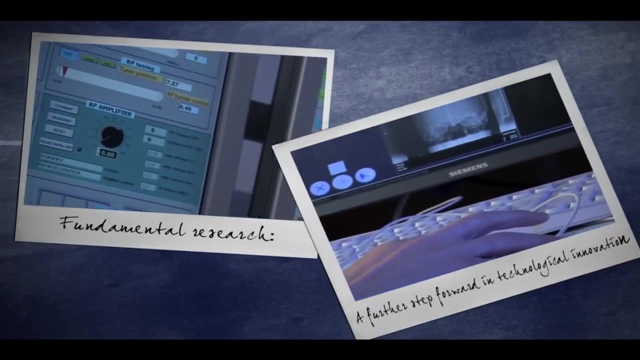 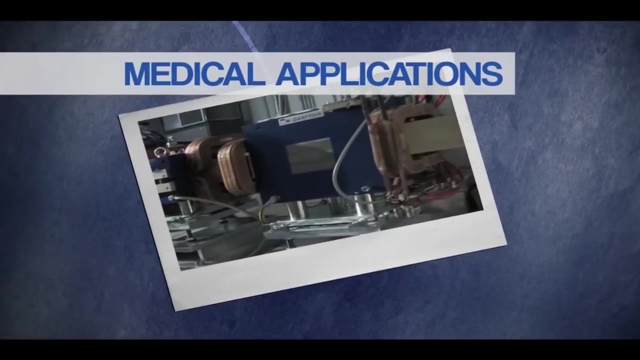 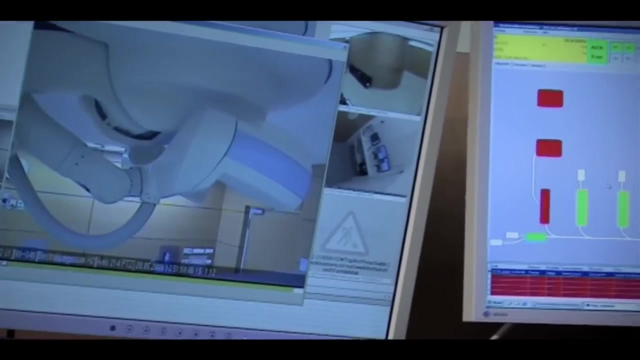 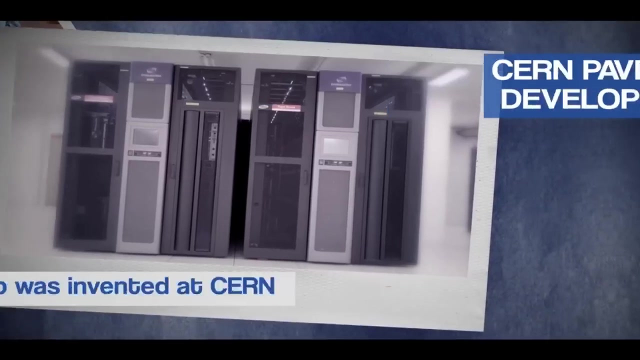 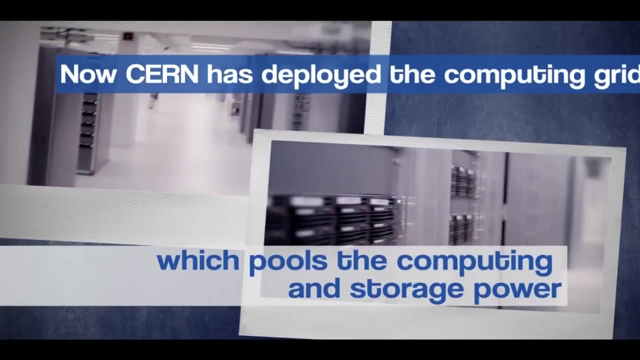 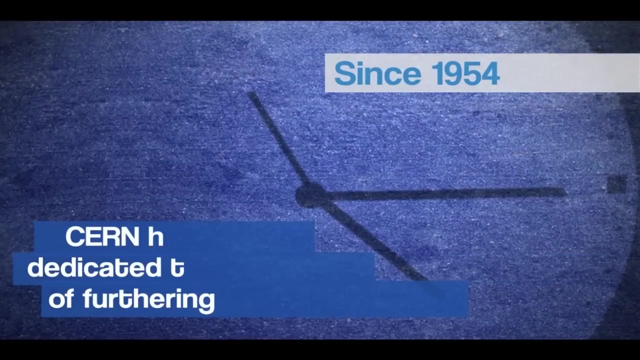 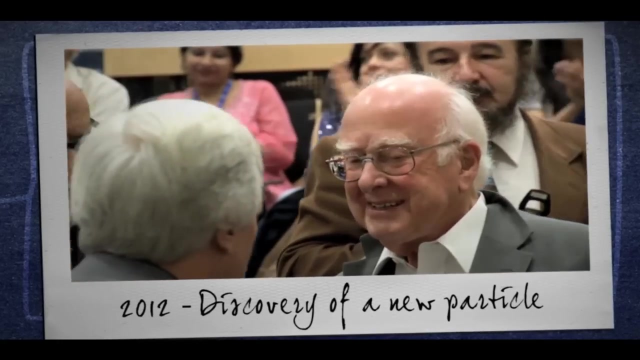 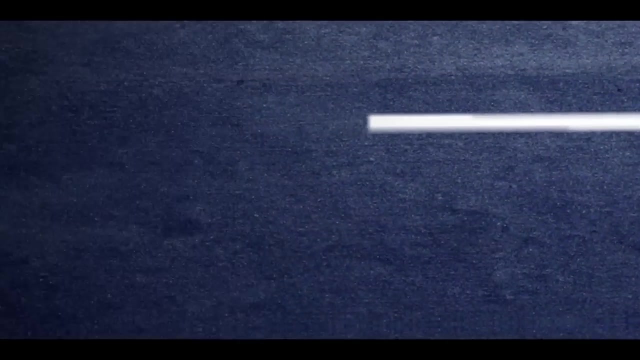 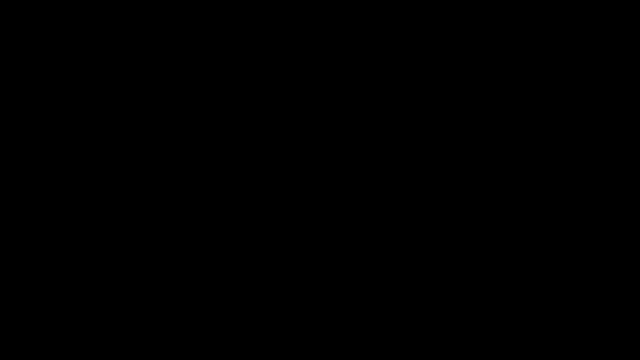 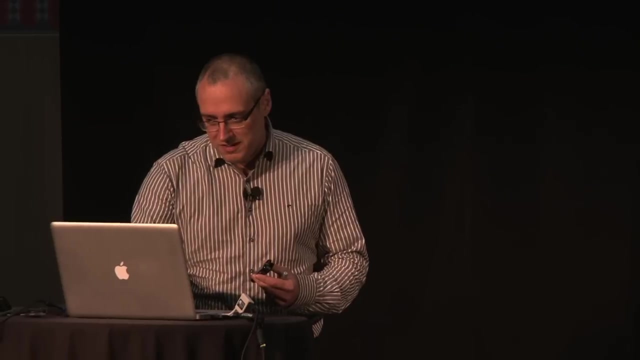 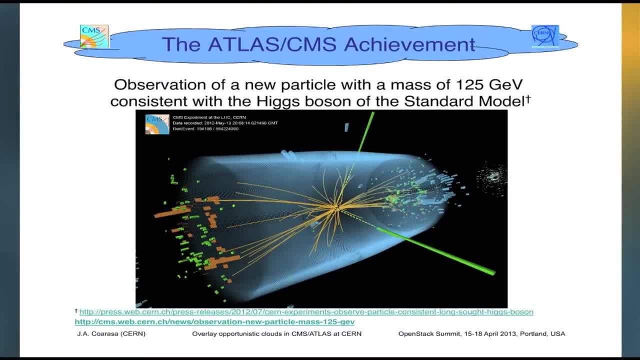 Skip a couple of transparencies, because this was in case Things were not. Now. this is what we discovered a couple of months ago, together with Atlas, basically, And we feel proud that, basically, after putting all of this effort, all of these people there, 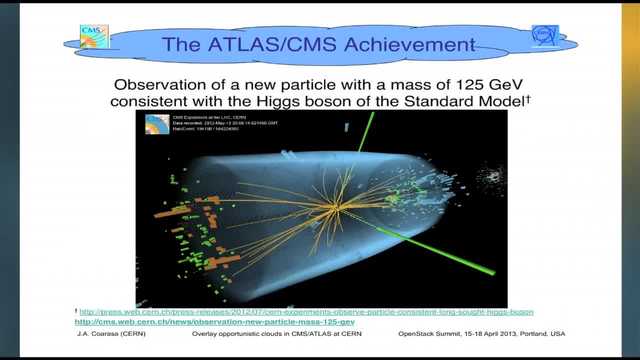 we could just see images like this one. Here you have basically a very similar image to what Randy was showing. This is a CMS candidate to the Higgs. So you have the protons coming this way and this way And if you integrate the energy of these two photons you see that it has this particular energy. 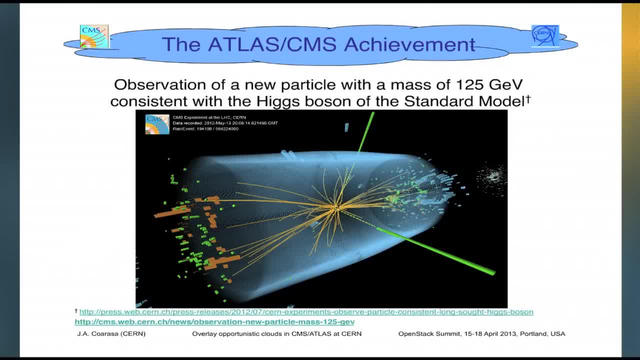 which is the mass of this particle Now, with just one single event? you cannot know, because there are many other events that fake the same picture here. But if you do statistics, and this is a, This is a picture from the statistic made by Atlas and I will not go into the detail. 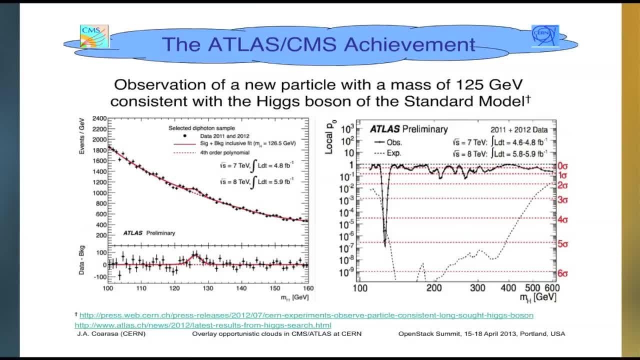 I think Randy already explained a little bit more what I'm going to explain. But basically what you see there, that there's a bump. This bump means that there is something at around the energy of 125 GeV. Okay, And this is statistically significant. 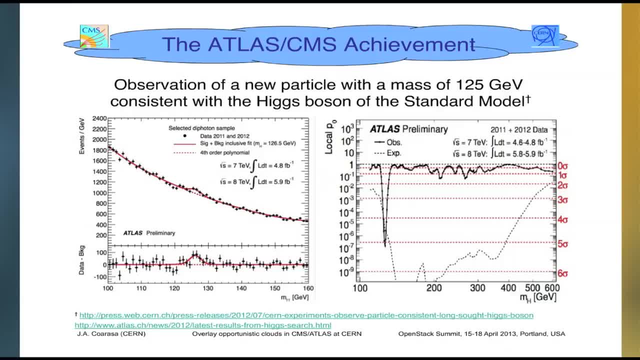 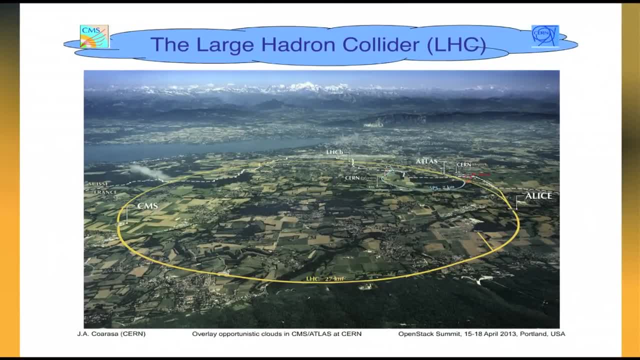 It means there is something new. We were expecting it somehow, But it's still something new that nobody had seen before. So I go away from this now and I come back to the LHC. I will zero in in the ore cluster, but starting from what we have there. 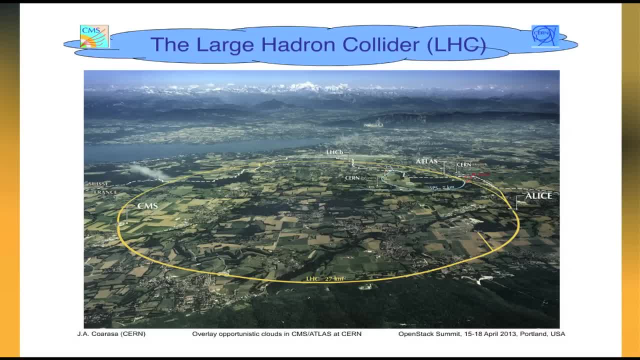 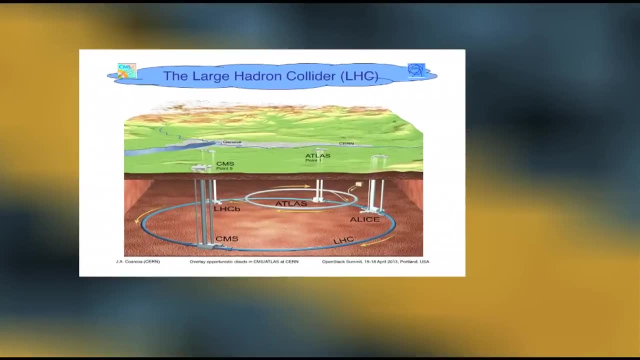 So this again is the 27 kilometers path of the particles inside the LHC, And there you have Geneva and the lake And you cannot see it, but there's the jet dough there And This is actually running around 100 meters. 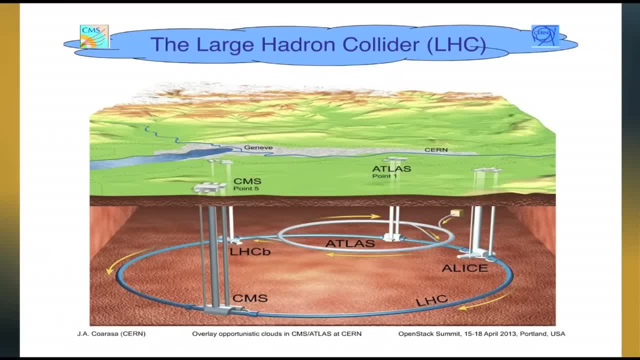 Below the Earth You have the four experiments ALICE, ATLAS, LHCV and CMS, And the protons will be injected in some smaller rings on the LHC until they get the proper energy, until they can basically sustain the. 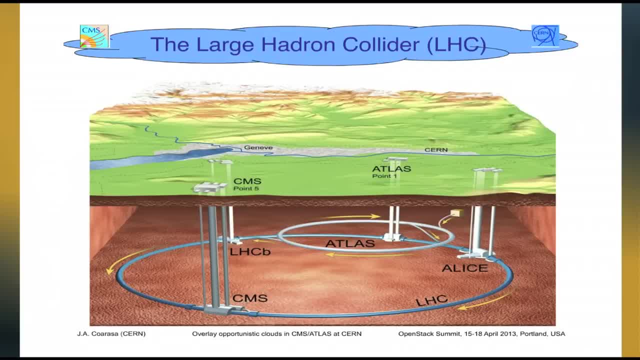 Well, basically you have to think that you cannot accelerate them right away to 7 GeV. You have to accelerate them in stages to the energy, and they can basically run in both directions, and then you can collide them in the four experiments you have. 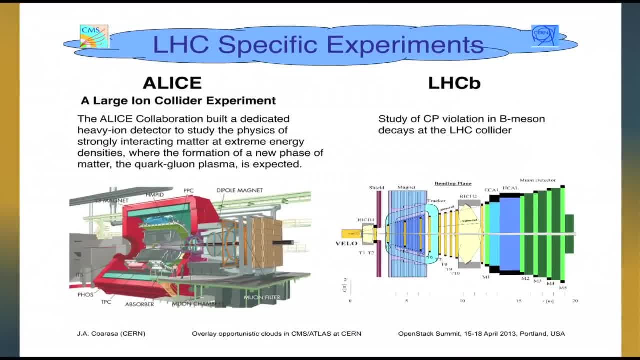 Now we have four experiments at CERN. Two of them are specific. They are made to study some specific physics. ALICE is made to study basically quark-gluon plasma that may appear out of collisions of heavy ions. LHCV is crafted to study the CP violation. 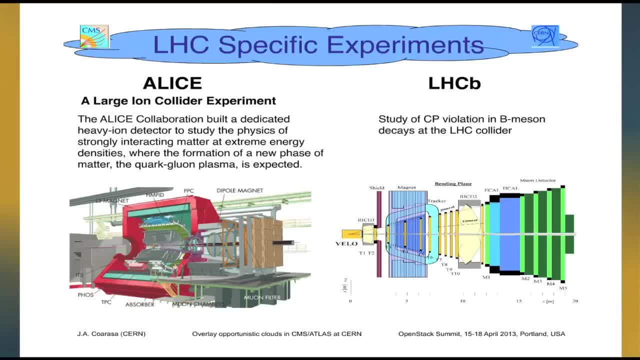 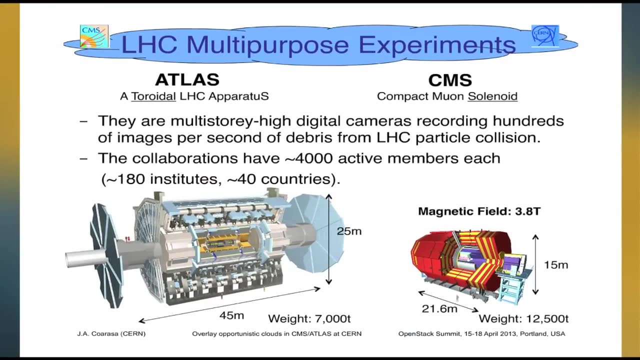 in the B meson decays. that basically will address this issue about why don't we see the antimatter and we see the matter, Okay. And then we have two non-specific experiments, multipurpose, which is ATLAS and CMS. 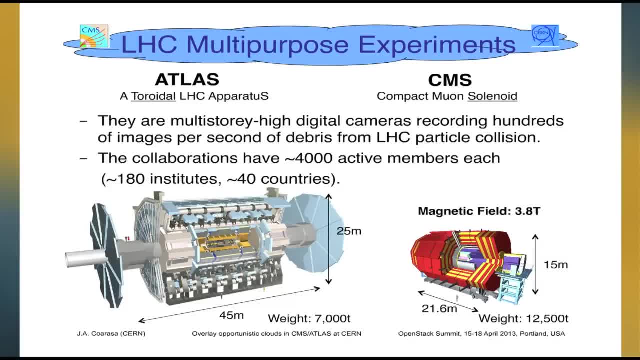 And you can see ATLAS is 25 meters. CMS looks much smaller. The reason why CMS looks much smaller actually is because we have one of the biggest magnetic fields on the Earth At this scale. we have it inside there And the thing is we wouldn't have these magnetic fields. 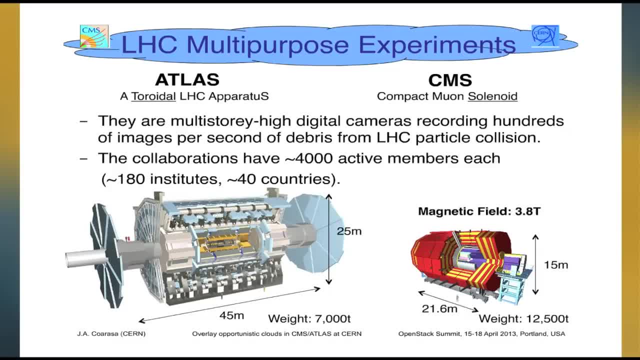 the particles wouldn't be contained inside the detector, so we could not be taking pictures of the whole event. Okay, so you have to imagine that the protons come this way and this way and then they collide, and then you have around 70 million channels. 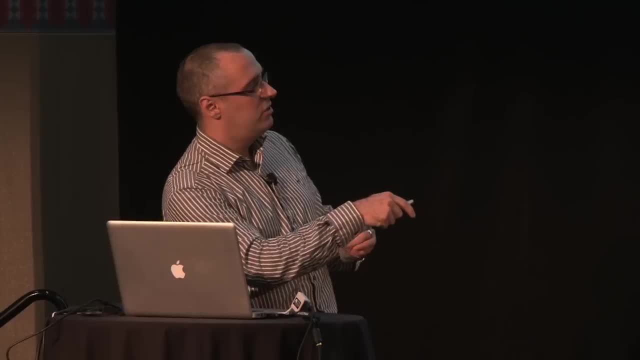 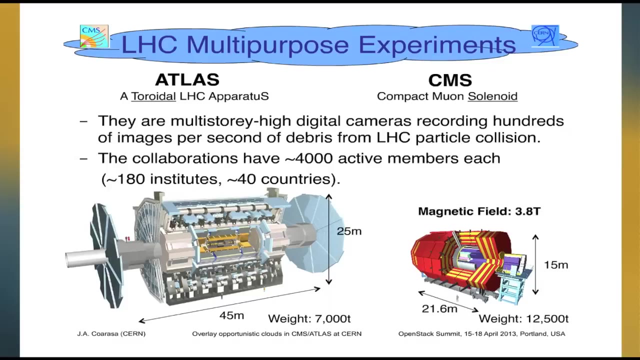 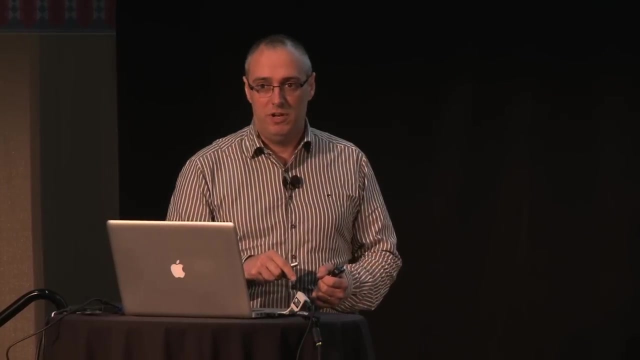 that come out of these detectors and you want to record the data from these 70 million channels. Now the particles will basically bend their trajectory due to the magnetic field and if they don't bend it enough, they will go out and you will not see them. basically, 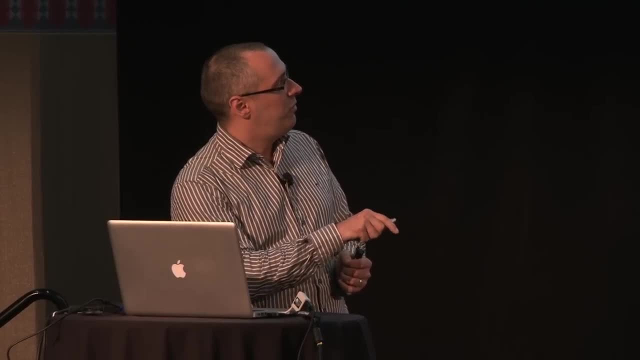 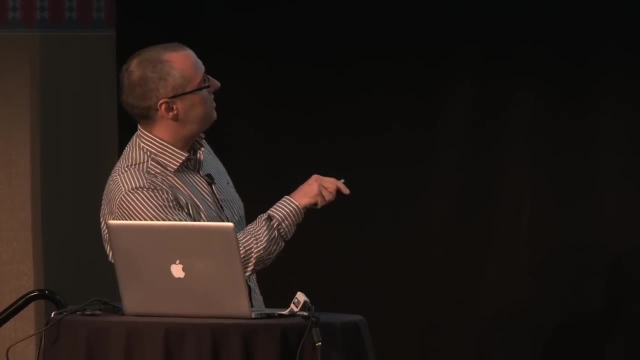 So this is why we are smaller, but we have a bigger magnetic field. It's a trade-off. This has good things and bad things. For example, you can walk inside the detector in ATLAS, but you cannot in CMS. If you have to fix something, you have to put the detector apart. 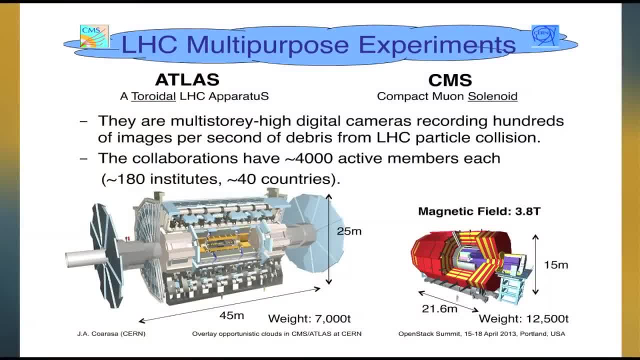 Okay. so coming back to the detectors themselves, you can imagine them, as Randy said, as big digital cameras. okay, with more than 70 million channels of electronics coming out of them. Now the collaborations are also big To build this thing. we are around 4,000 people in each of the experiments. 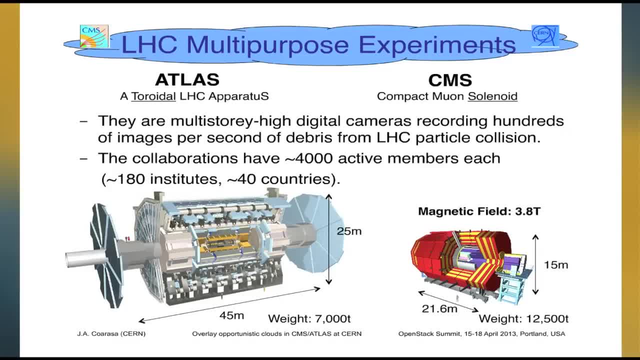 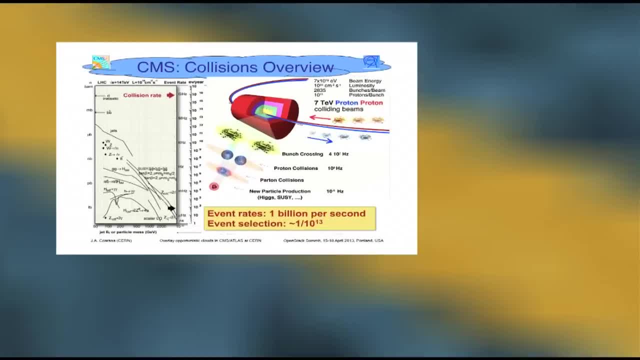 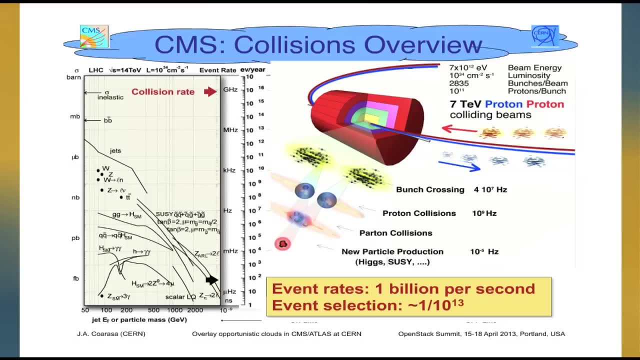 active people and we involve more than 40 countries and 180 institutes. basically, Now, what happens when something collides First? we're interested, as I said, in only a few of the events that happen. We know most of them, okay. 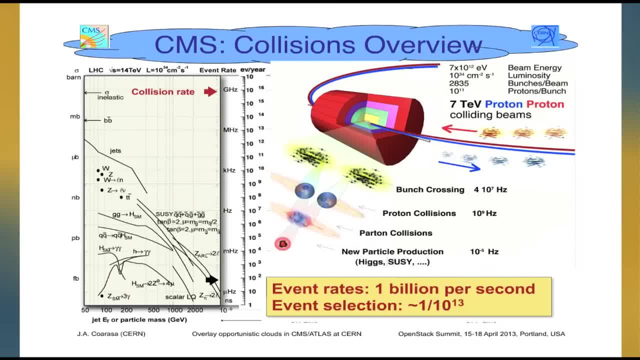 So here you have. this is. I'm not going to go into the detail, but this tells you that we can predict a lot of what's going to happen when two protons collide. okay, And we're interested in the things that we haven't seen. 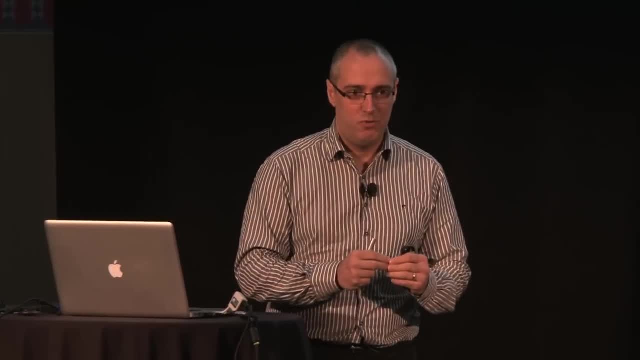 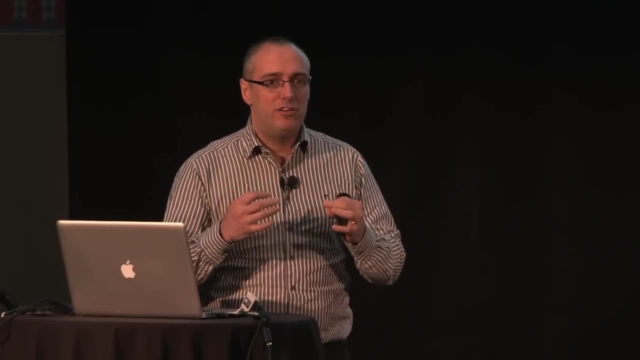 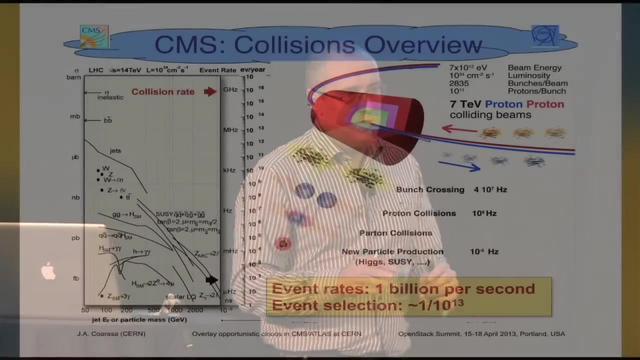 or that we cannot predict. So far we could predict, for example, the Higgs, And let's go to the numbers to see a little bit later. why do we need the computers we need? We have branch crossing every 40 millions of a second. okay, 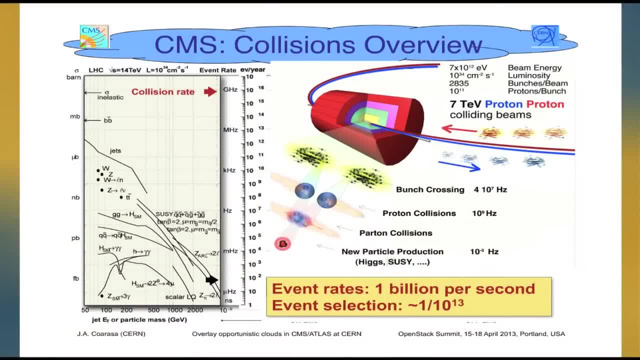 We have 40 million crossings. every second Out of these crossings, there is many protons going into each other and some of them will collide- Not just one, but some of them will collide with each other, which means we don't have 40 millions. 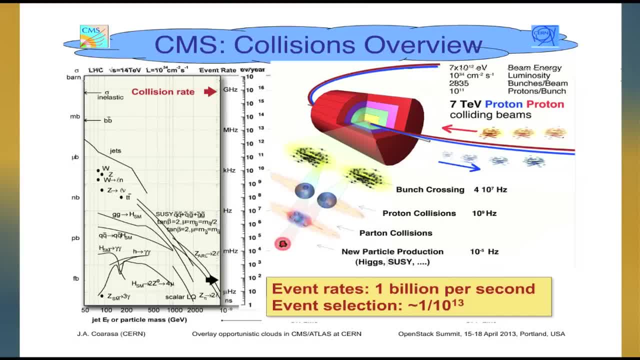 but we have more a billion of events every second. Now, that's a lot of events, okay, And we cannot record all of it. Also, we are not interested in most of it, Actually, we are only interested in basically. 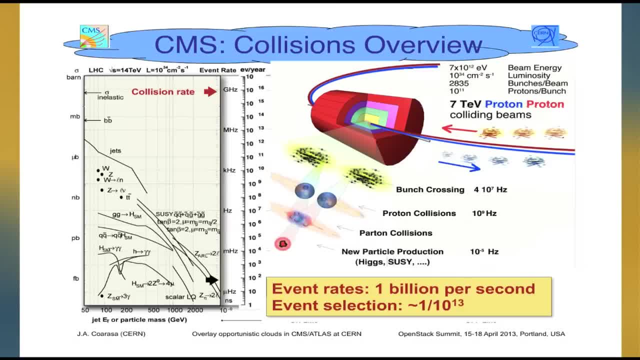 one out of 10 to the 13 events. Every 10 to the 13 events, there will be one that we may be interested in. okay, So we have to select it. How do we do it? Okay, we need computing power. 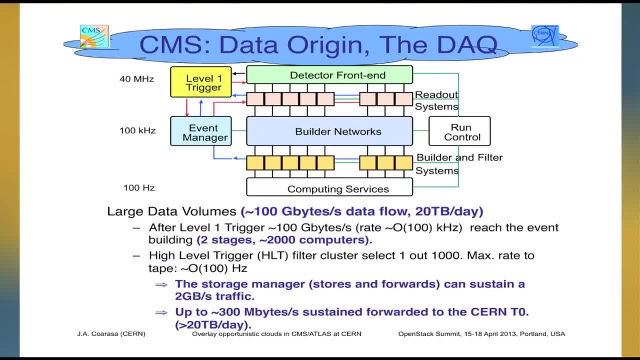 Now this is the CMS data acquisition system. The first part up to here is composed of electronics that has been designed to work, So basically cope with 40 hertz. After that, after the event manager and the builder networks. all of this is of the shell computing elements, okay. 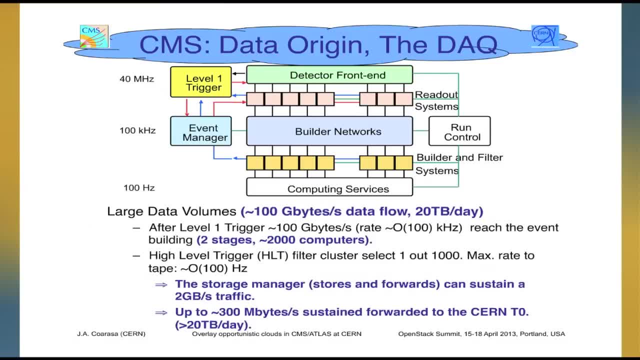 And when it was designed it was like, basically eight years ago or nine years ago, This part up here could not be done with computers. This is why it was what it is, basically Something crafted for us. Now, part of this could also be done in computing. 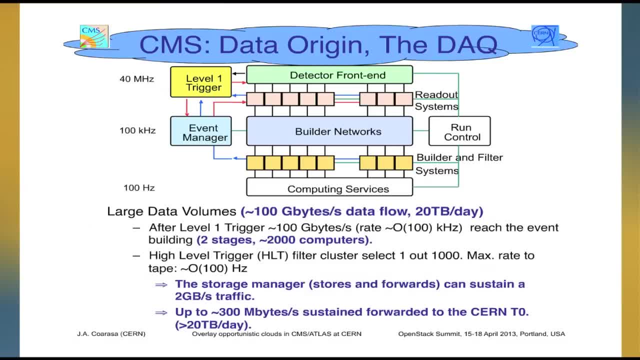 but at the time it could not okay. So we also have only one level of trigger or level of selection of interesting events in electronics. The second level, or the high level, is actually off-the-shelf computing, And through that off-the-shelf computing 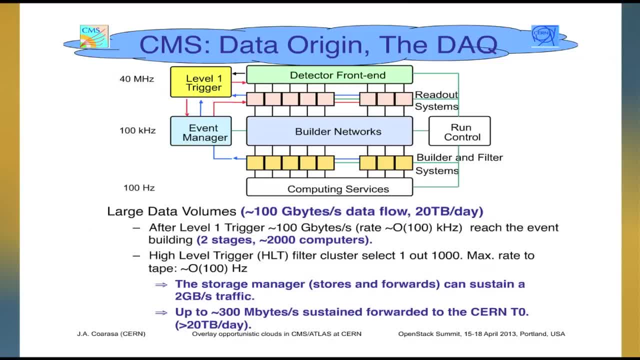 we have basically around 100 gigabytes per second of traffic to our networks And then they will select our computers. some of the events that are interesting. Basically, one out of 1,000 is selected and we throw it to the storage manager. 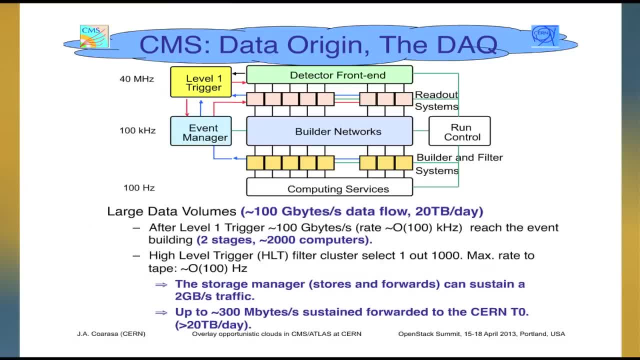 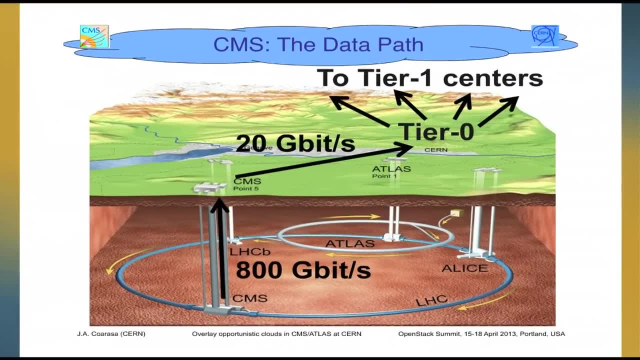 that will store it and forward it to tier 0 at CERN for later analysis. okay, Now this is the path of the data. again, We have 800 gigabytes going up to the surface and from the surface to tier 0 at CERN. 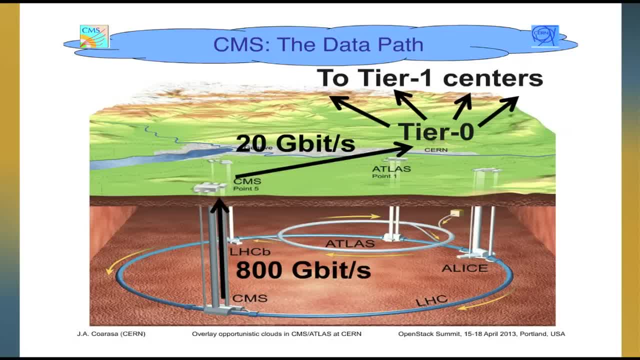 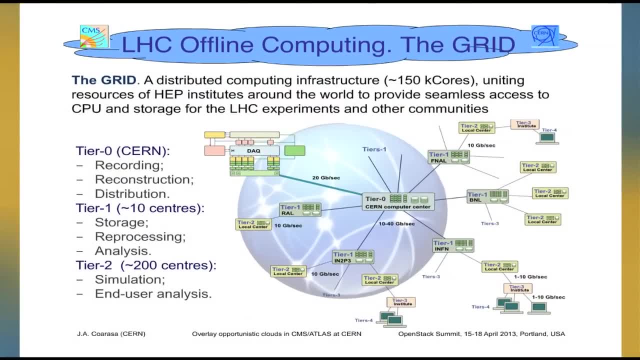 there is 20 gigabytes- 20 gigabytes, sorry, per second- And from here it goes to the tier 1s. At the time that this was projected, it was basically impossible to have the computing power needed in just one place. 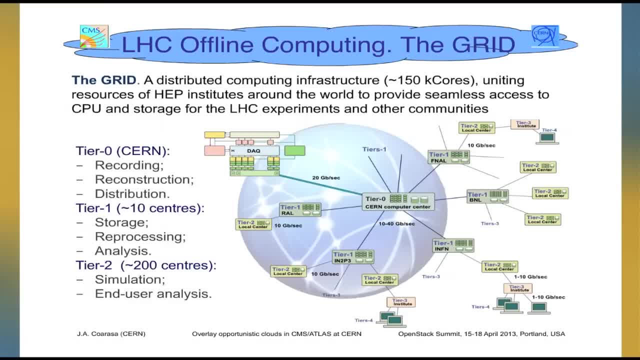 So the high-energy physics community crafted something we call the grid, which is a distributed computing infrastructure that unites many high-energy institutes around the world And provides basically access to computing power all over the world. It's designed in a tree level. 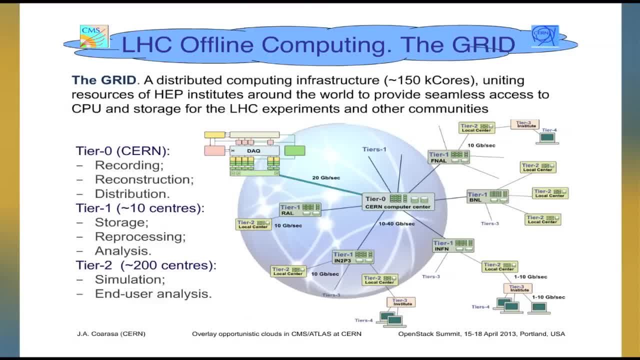 So we have tier 0,, which is responsible for recording, reconstruction and distribution of the data, And there is the tier 1s, which we have around 10, and it's storage, repositioning and analysis what they do. 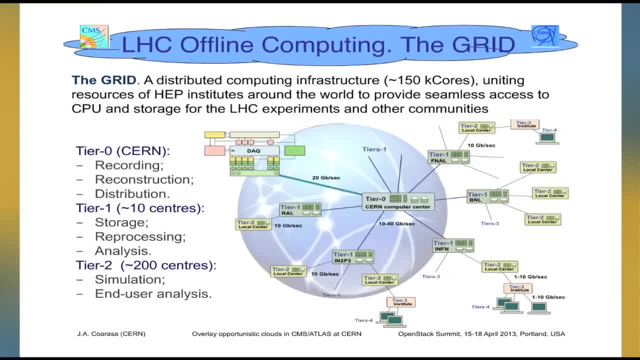 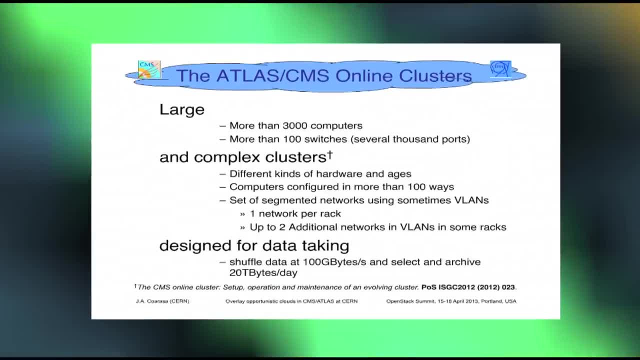 And then we have another tier 2s and tier 3s that will do the rest of the job. Now, keep this picture in mind, Because later I will be referring a little bit to it. Now, all clusters, as I said. 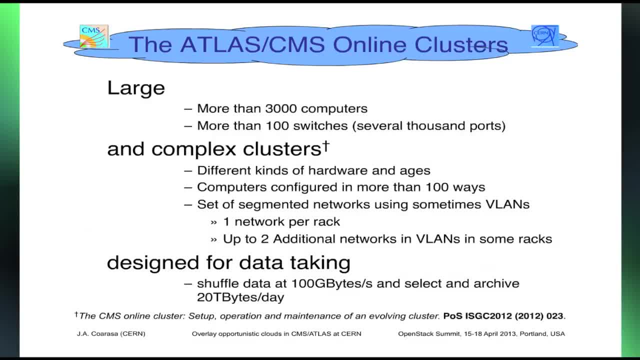 have a cluster dedicated basically to data taking, to select part of the events that we want or we think that will be interesting for later analysis, And we send these events to CERN. So we have a large and complex cluster. Complex because actually, 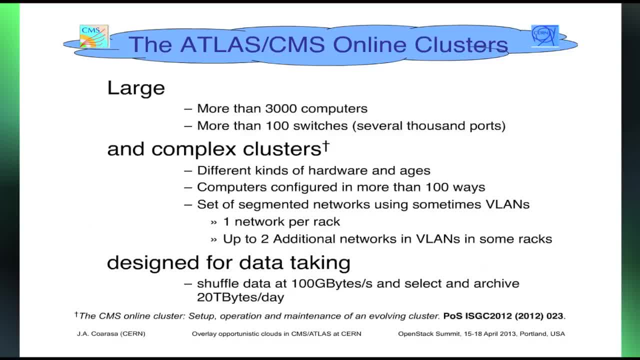 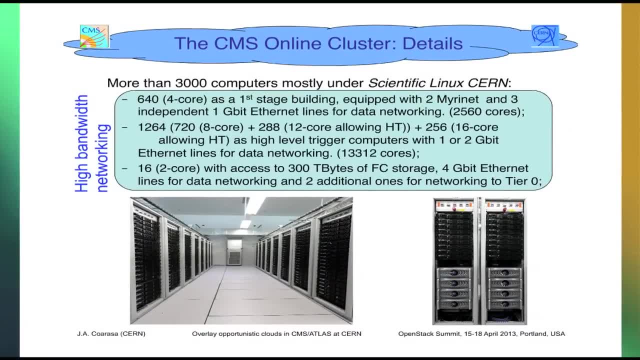 the control of the experiment itself is quite complicated And it has been basically designed for data taking, Nothing else. OK, Even so, we have many of the things that the industry has there, like databases, et cetera. I'm not going to go into detail of how many computers and so on. 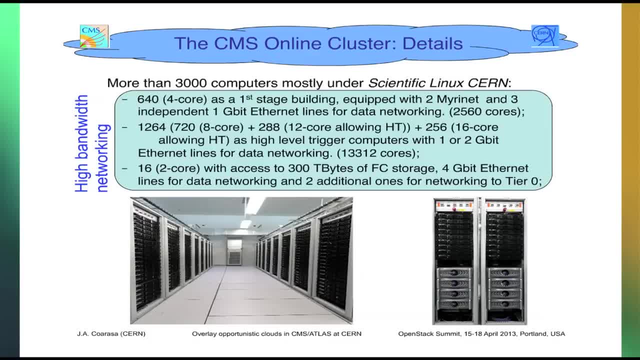 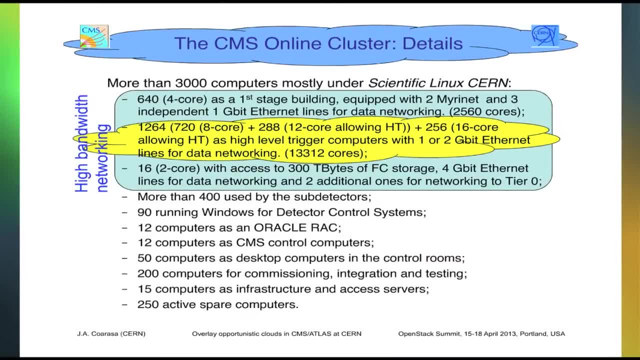 This is only for somebody that wants to have a look at it. OK, I don't know why it's not going on. OK, Now, what we did is we cloudified this part here. This is basically the highest level trigger computers. 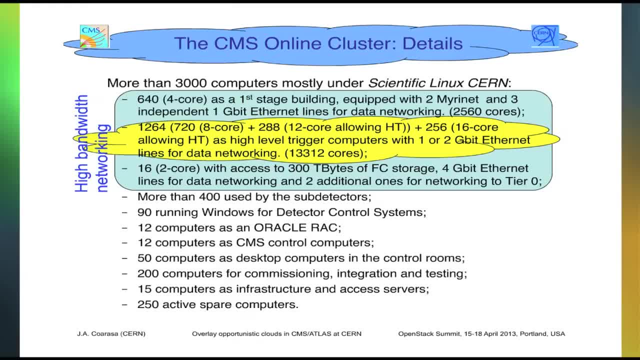 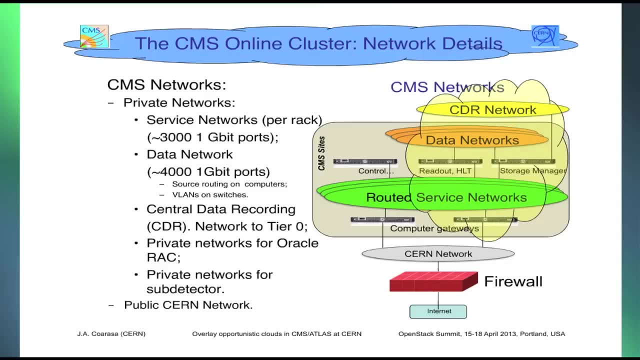 These are the newer computers, These are the computers that have high bandwidth to CERN And actually the computers that make sense to do something with them because they are the most powerful computers. About the networks, we are also kind of not easy. 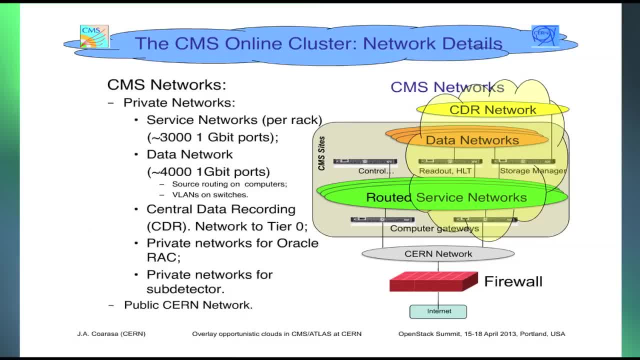 We have basically. so that's the firewall connecting us to the internet. This is our CERN network And this is the CMS experiment. We have computer gateways that connect to the CERN network And this is one gigabit link, And then we have every rack that is connected. 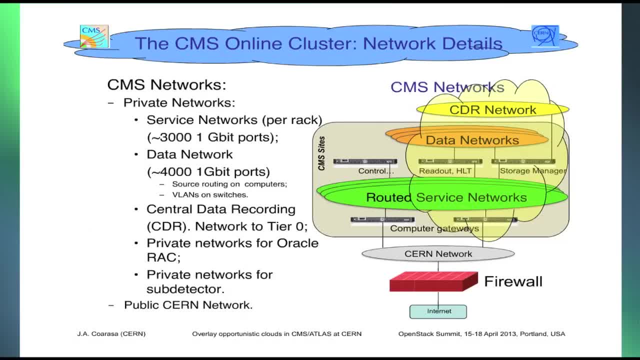 to our internal rooted service network. All computers are connected to these networks here. OK, And then this is the HLT computers I was talking about. The HLT computers are also connected to what we call the data networks. Every computer has a one gigabit at least, maybe two gigabits. 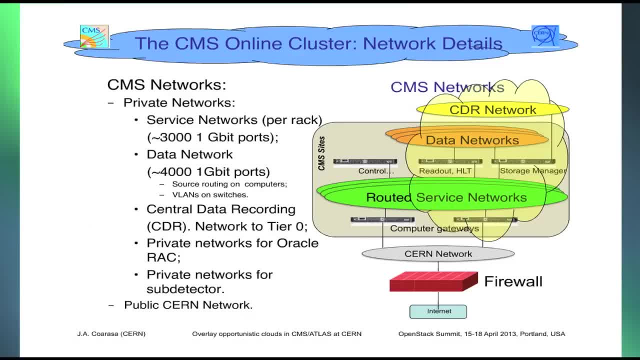 or maybe three to these data networks, depending on the power of the computer, And they will be connected to the storage manager that may be throwing the data to the TR0 through these 20 to 40 gigabits per second link. Now, in reality, all of these may complicate. 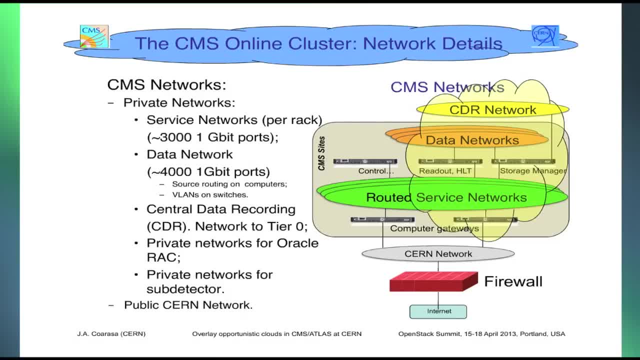 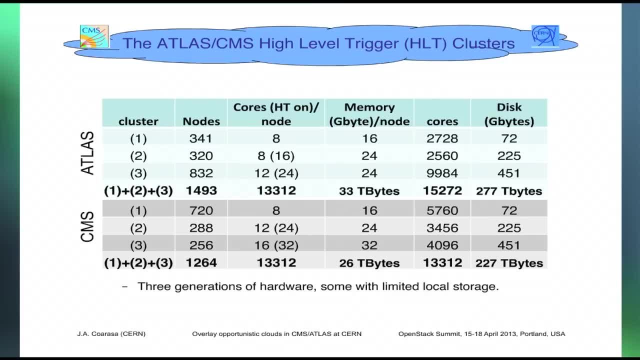 all deployment of networking, as you will see later. OK, So just for reference, We have around 1,300 computers, 13,000 cores And Atlas has a similar farm. basically Some of these computers like the first generation. 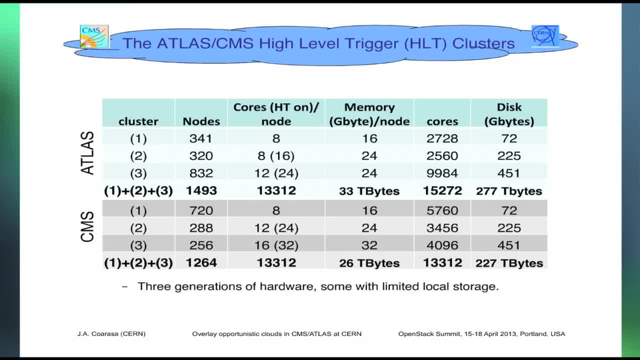 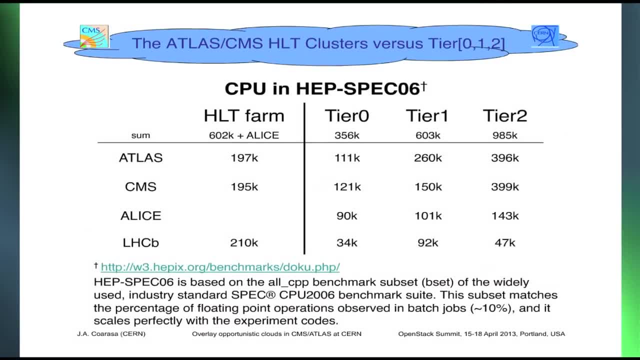 don't have a lot of local storage, which may be a problem for some of the things we want to do. Just remarking this. Now, how do we compare to all this structure of tiers 0,, 1,, 2,, et cetera? 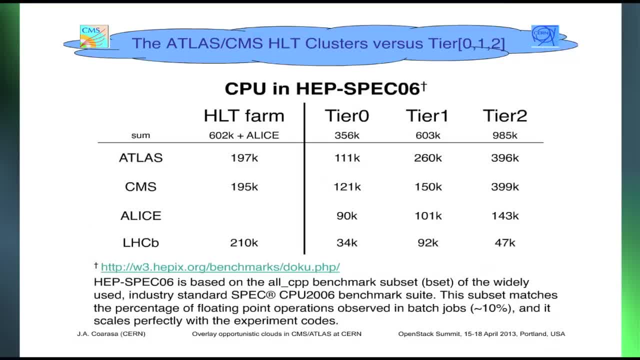 I'm going to use this HEP spec, which is basically related to the spec CPU 2006.. And basically it reflects how well all software will run on a given computer. But just bear in mind, it's a quantity that tells you how fast the computer is, and that's it. 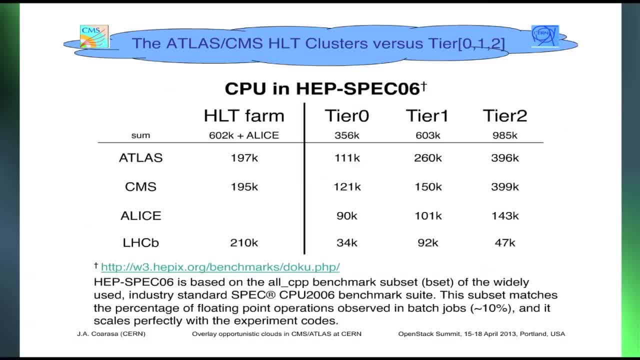 So how fast our computers are at CMS online farm. this is 195 kilo specs And the tier 0 itself has 121.. And the tier 1s in total the ones dedicated to CMS, because there are tier 1s dedicated to CMS. 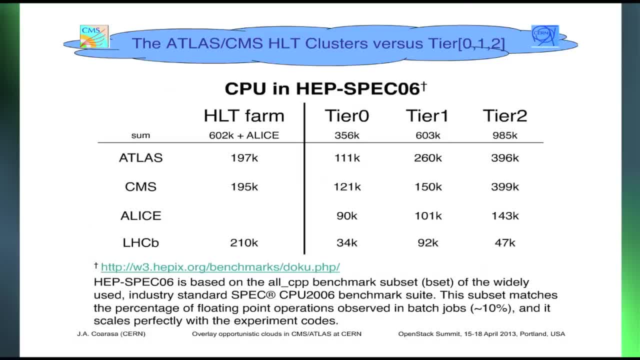 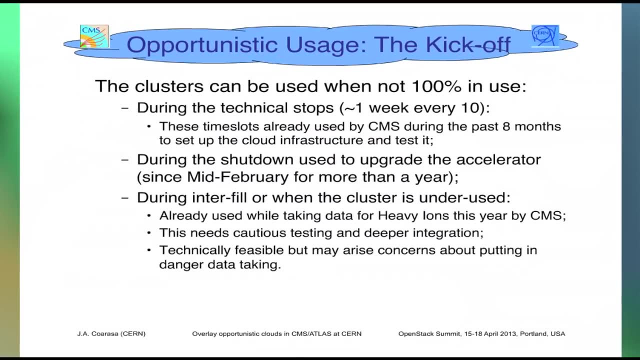 others to Alice, et cetera, et cetera. there is 150.. So we are 1.5 times of tier 0, basically, Now the question comes: there's no money now out there. People want to, or need, to update their computers. 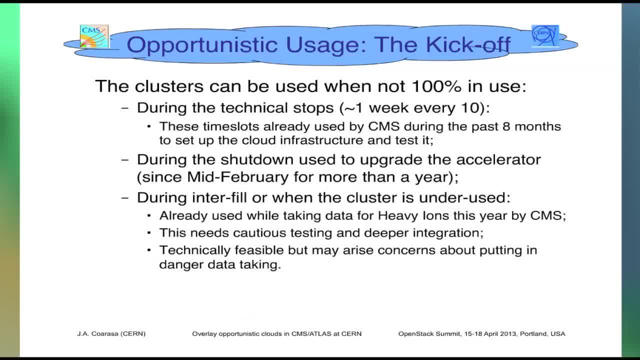 or update their computing gear, basically to be able to analyze more data the next year, Because every year we take more data. So funding agencies came and said you don't use your computers sometimes, right? No, we take data half of the time. 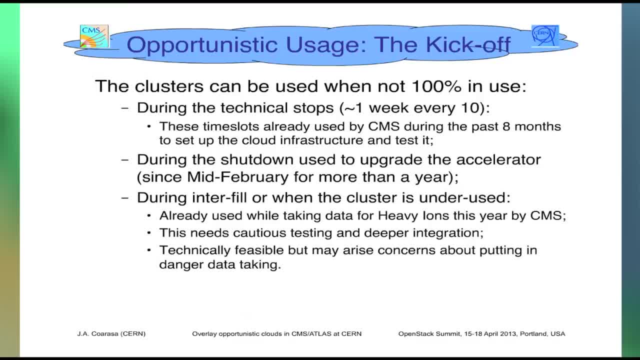 So why don't you actually use them? And then this is why we developed what we developed. Basically, we already did it. We already used the technical stops that we had- This is one week every nine or 10 weeks- to be able to deploy the cloud infrastructure. 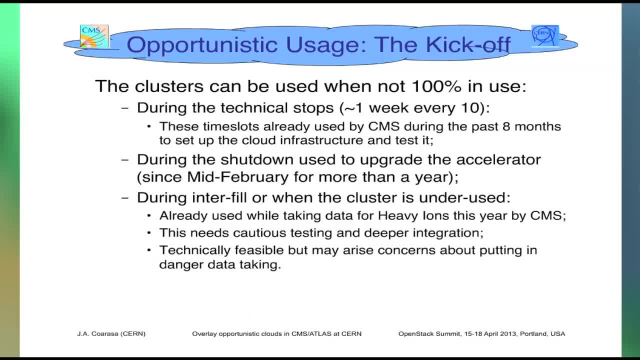 So we were deploying our cloud infrastructure when we were not running And you will see some of the kicks about it later. And, of course, we are using our cluster now in cloud production because we are not running for the next year and a half. 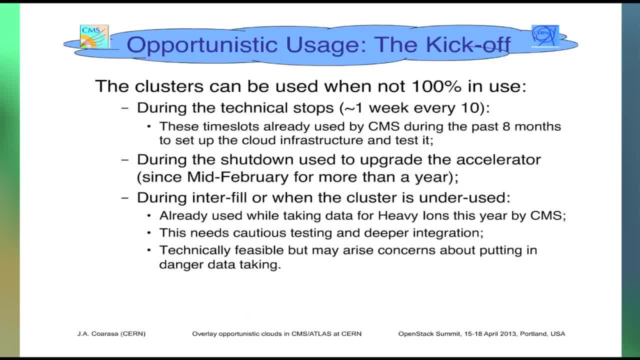 And also in a more aggressive way of using it in an opportunistic way. we could basically run our cloud when we either don't use it- we don't use our computers fully- or basically we don't use it because in an interval period, 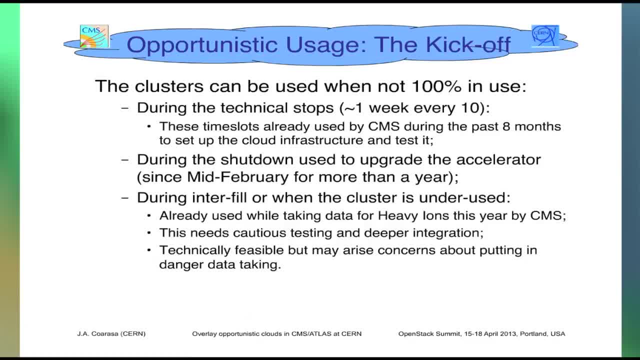 basically, we don't need the computers for anything. Of course this is a little bit more dangerous. We've done it already. We did it from January. We ran a third of our cluster. We ran a third of our cluster in cloud mode. 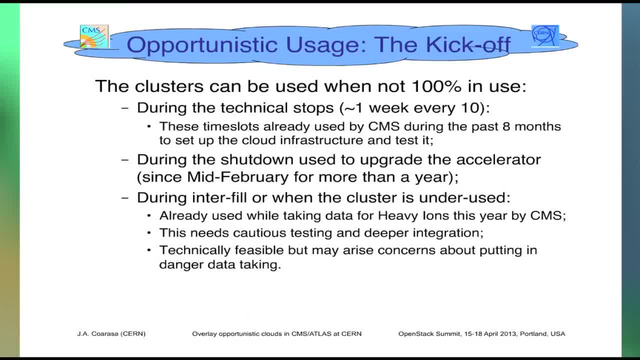 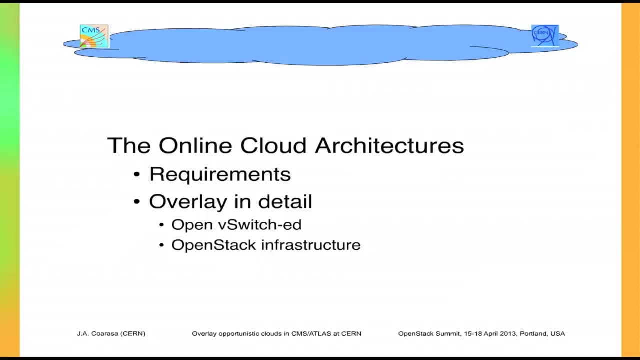 because the two-thirds were enough to take the data, But this raises many, many, many internal problems, maybe, if anything happens. So far nothing happened, So nobody's basically saying anything against this effort. So what are the requirements for our cloud? 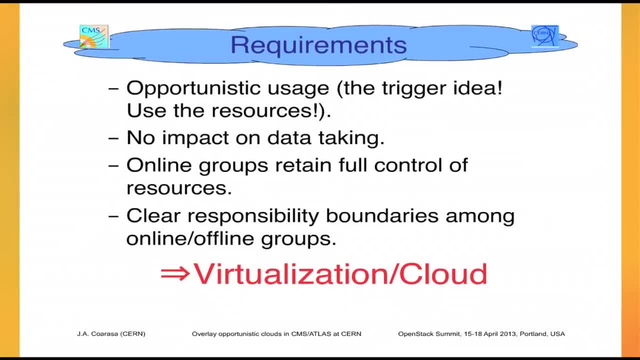 And why did we choose an overlay mode? OK, the requirements are kind of clear. We want it to be opportunistic. Our cloud should be used, and can be used, any time that we don't use the computers. Of course, it has to have no impact on data taking. 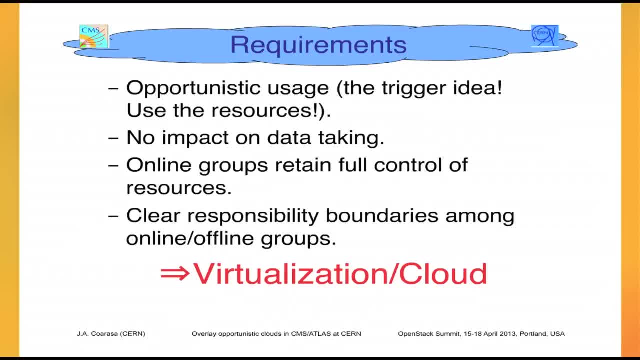 The online groups, which is, in this case, us, should retain full control of the resources, And there has to be a very clear responsibility boundary between the online and the offline groups. The offline group is basically our client, OK, And this is one solution to all of this. 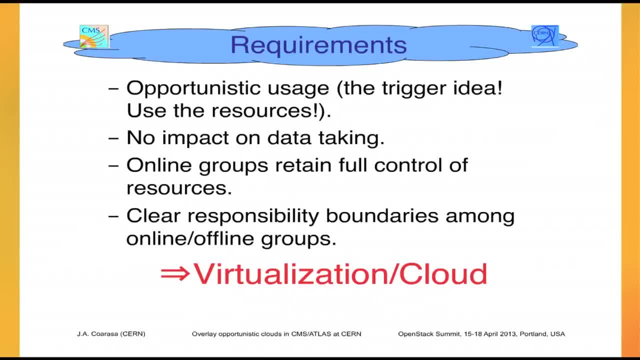 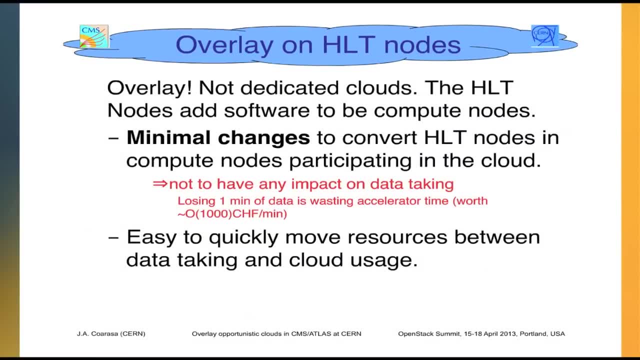 is basically virtualize and put the cloud on top. That's it. That's a very easy way of doing all of this. Now we actually chose also an overlay. What do I mean by an overlay? Our computers. we use them as they are. 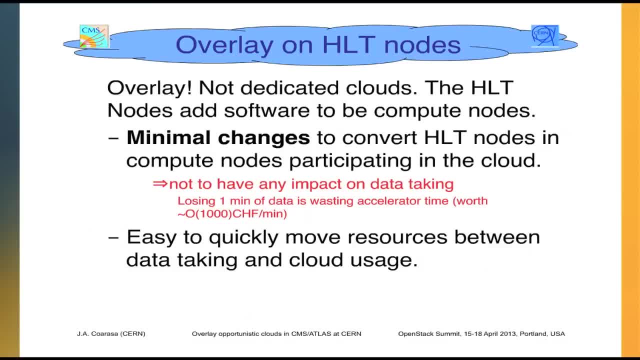 They have their software. We don't touch the software. They have to do the data taking, But we deploy on top something that will look like a cloud that people can use. So actually we run on the bare metal. Our data taking runs on bare metal. 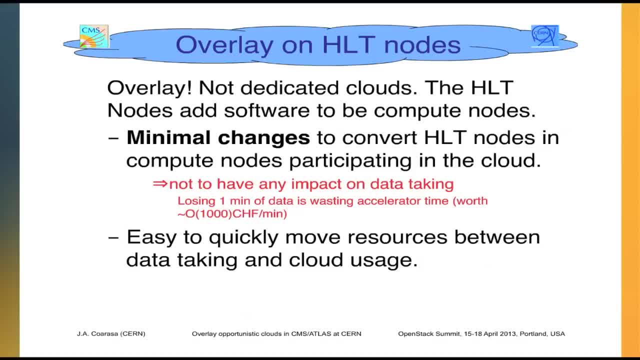 It's not cloudified or virtualized or anything, But on top of that we put a layer so that people can use our computers. OK, Then we did minimal changes to our computers. We just added a couple of things, And it's also easy to transfer all resources. 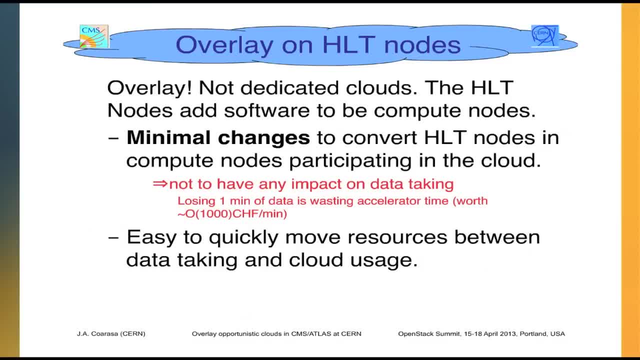 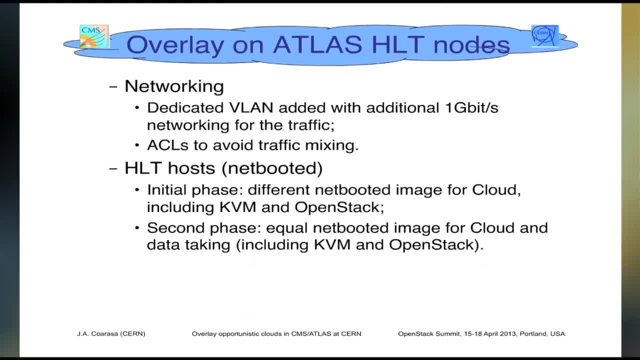 from being used to data taking or being used to actually cloud. Now, what did Atlas do? I'm talking fundamentally about CMS, because I know it better, Because also we started a little bit earlier, But now what they are doing, or they have done already- 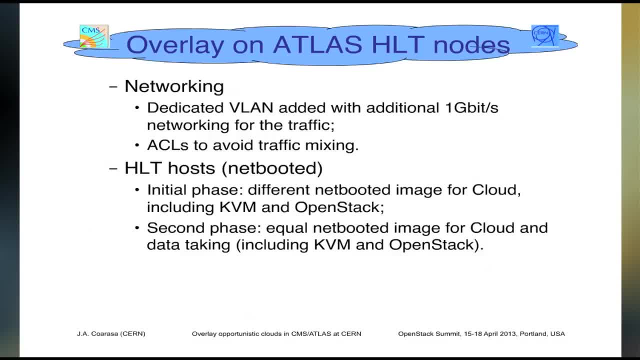 is in a test bed. They just deployed a new physical network together with a new villain, so that the traffic of the networking will not touch the data networks at all. OK, This is about what they did for networking And for the HLT hosts. what they are doing right now. 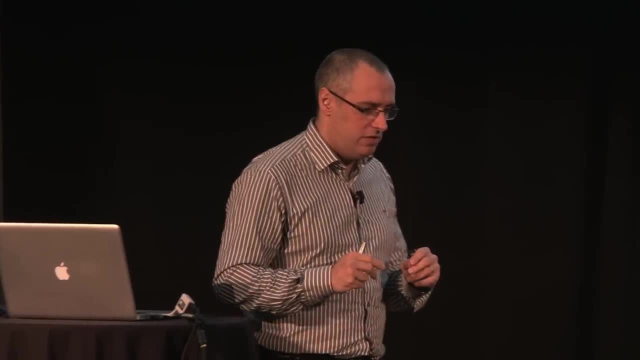 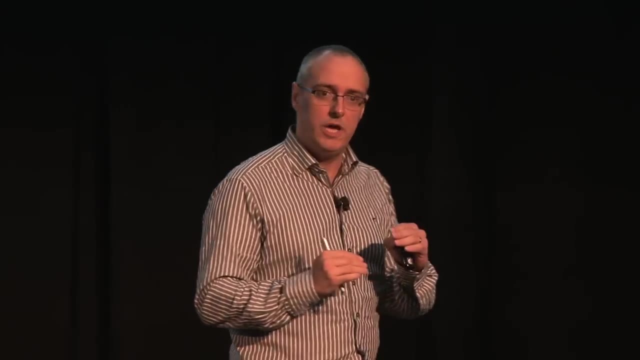 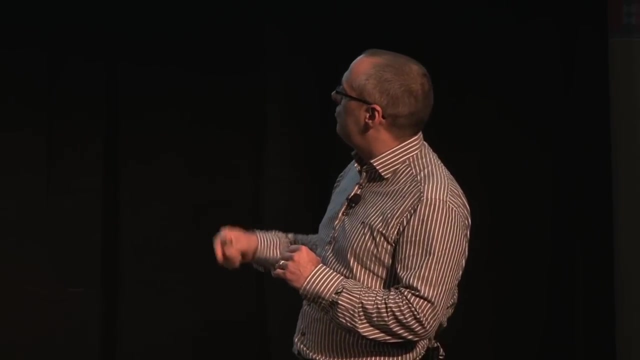 since they have an HLT farm that they network. they are having a different network and they have a different image from which they network their computers. OK, So that they can run the cloud or a different one to just run data taking. In the future they will have the same image. 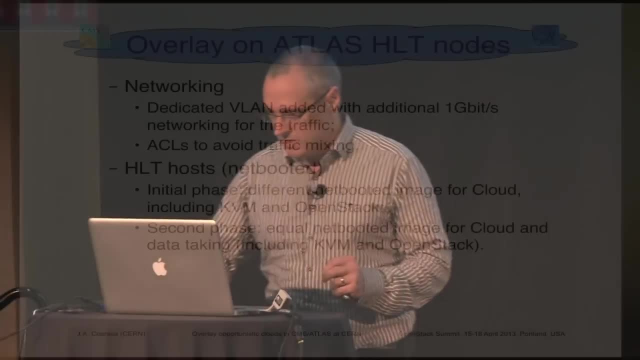 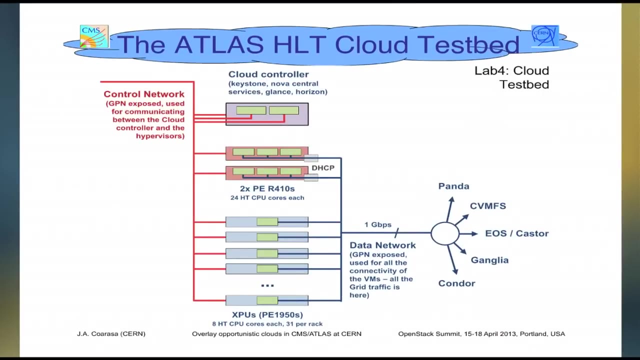 But now that was the easiest to do. Now, what did we do? And I will go OK, this sorry, This is actually how does it look like for Atlas now in the test bed They have individual one gigabit links of the computers. 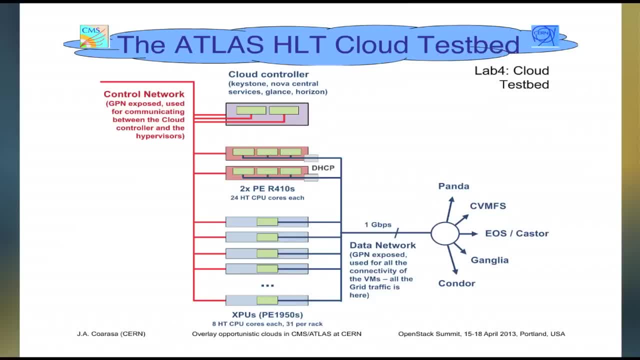 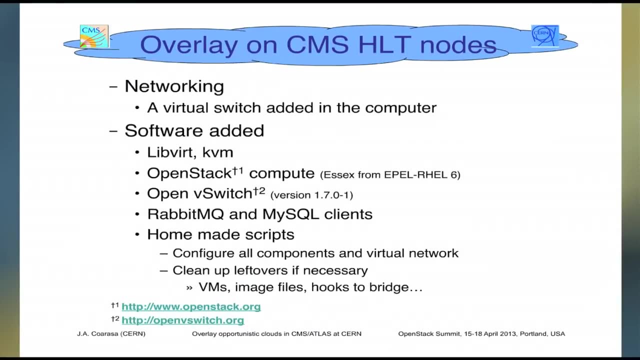 This is a rack. They have a cloud controller in the rack for the cloud And basically this is the one gigabit I was explaining. that goes to the data networks, et cetera. Now how do we do it, Since we were running and we couldn't touch actually, 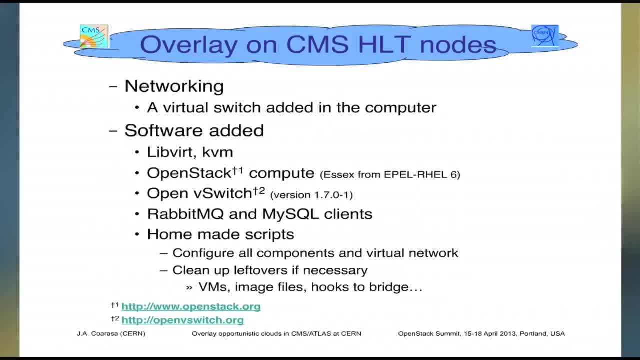 the networking. no adding villains, no adding anything. we couldn't do what they did at the time. So we added a virtual switch to each computer. I'll go into more details in the next transparency. And then, as of software, we just added the KVM virtualization. 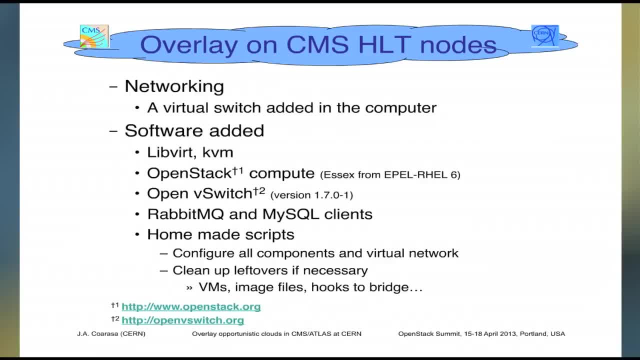 layer, the OpenStack compute to every single HLT node, the OpenV switch and then the Rabbit and MySQL because of dependencies, and some other scripts to automate the things like configuring, et cetera, and also to clean up because sometimes some things go wrong. 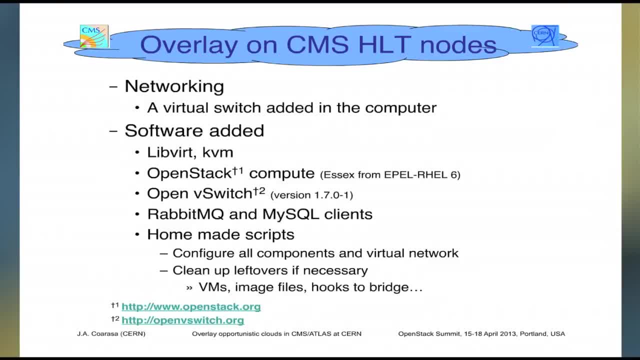 or VMs get stale, The connection to the basically switch stays but the VM goes away, and this kind of thing. So we added some automation that will run every 15 minutes and will clean up things since things were left there. Now about the networking, we had to do a little bit more. 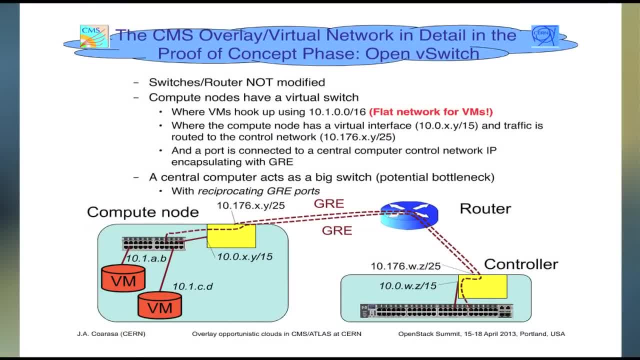 I mean, this is not standard among the clouds, I think. So we couldn't touch the routers or the switch, We couldn't add VLANs, We couldn't do anything. But what we did is we, as I said, we have a virtual switch in every single computer node. 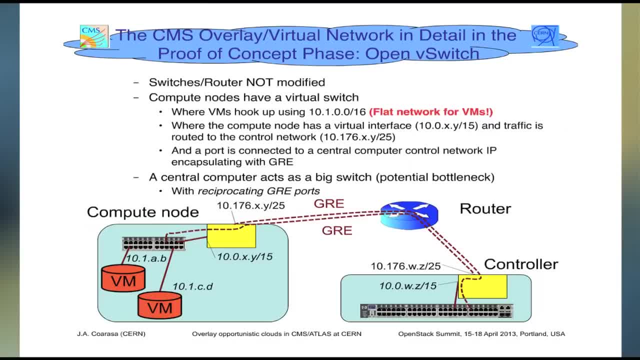 All the VMs will hook to this switch And the compute node has a virtual interface too that is in the same address space of this And actually, through routing, this virtual space is connected with a gray port, basically a GRE encapsulation port that goes from here: 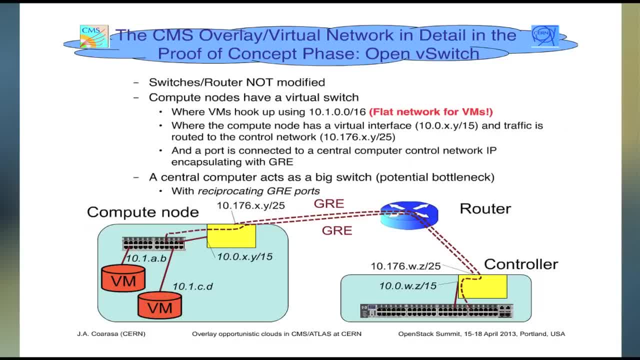 to our very big virtual switch in the controller. There is another one going back And basically what you will see after this is that all the VMs are living in a 10.1, or real addresses is 10.176.. All this traffic is encapsulated through these addresses. 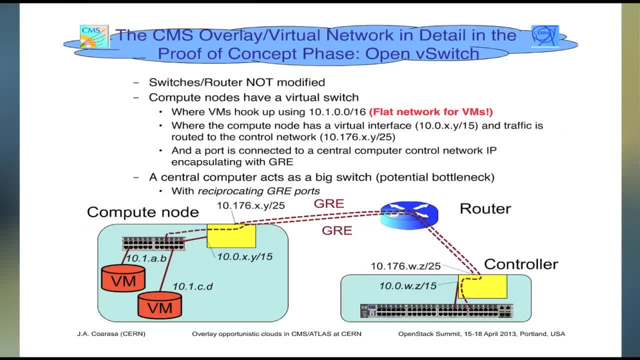 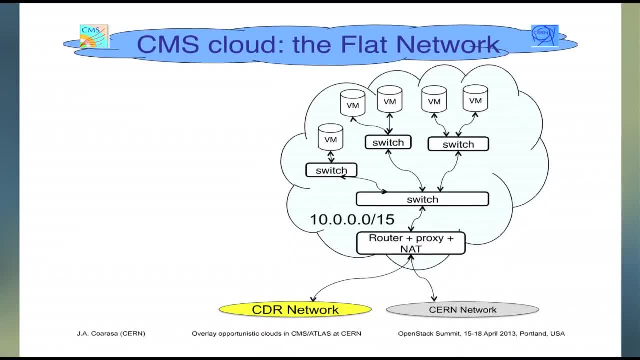 So all the ACLs et cetera don't kill our traffic at the router. OK, And in the end for the CMS cloud there is a flat network simply. So we use flat network with NOVA network From the point of view of basically cloud. 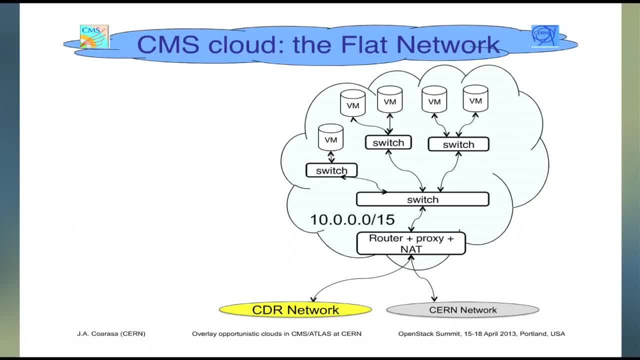 it's very simple. At the other level it's not that simple, But anyway it was not that difficult to implement And as a proof of concept- because we were in the proof of concept without touching anything of networking, that was basically. 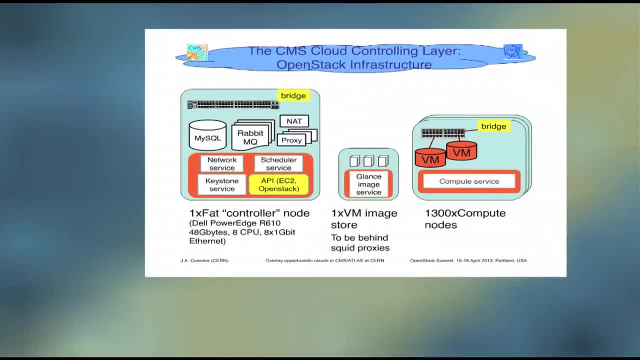 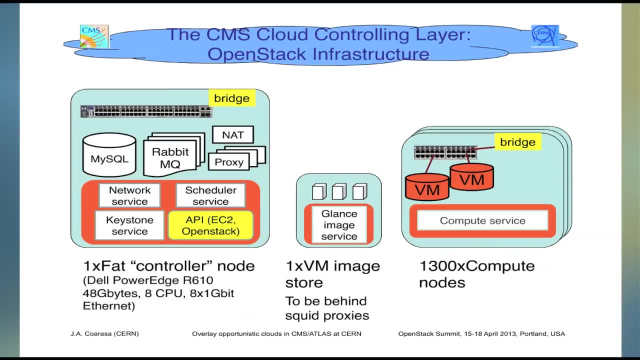 what allowed us to continue. OK, As of controlling our cloud, we deployed OpenStack. We have a FAT controller. All of this is based in Essex And you see the different services that we have: MySQL, Rabbit, The services of OpenStack that we run. 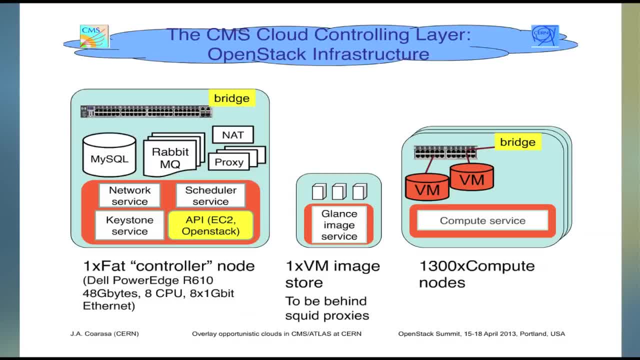 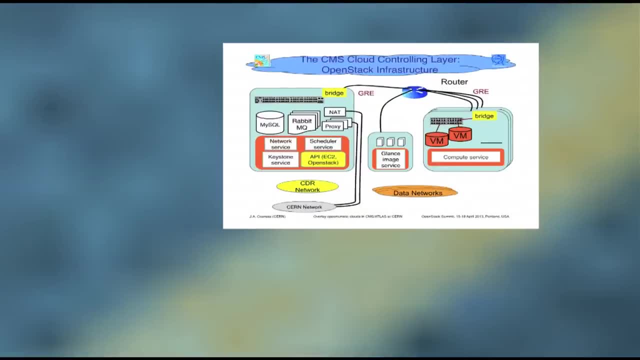 is the network service, the Keystone Scheduler and the API using EC2 and OpenStack. All of this is based on the NOVA APIs, And then we have our 1,300 compute nodes and one GLAN service. OK, That's pretty easy, actually. 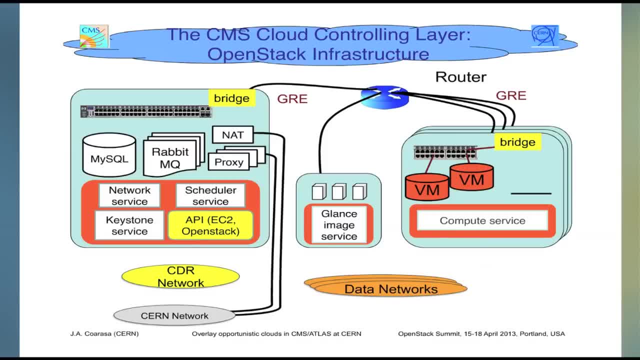 Now this is how it looks like when you put all the connections in place And you see that now, right now, we are not still using the connection, the big connection to CERN, or the data networks at all. We are all going through NATing and proxies. 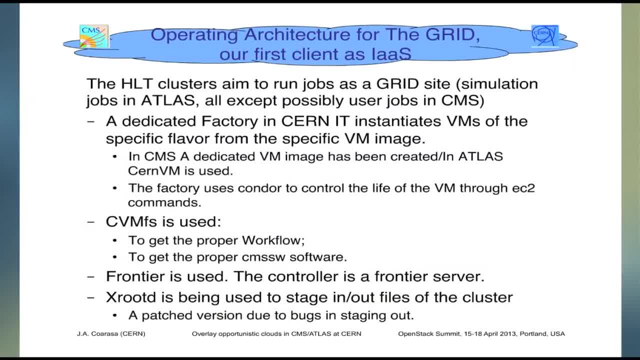 in the network, which is limited to one gigabit. OK, Now our first client is basically the grid. We should resemble a grid site, But for this we had to do some glue here and there. Actually, we have to have some services. 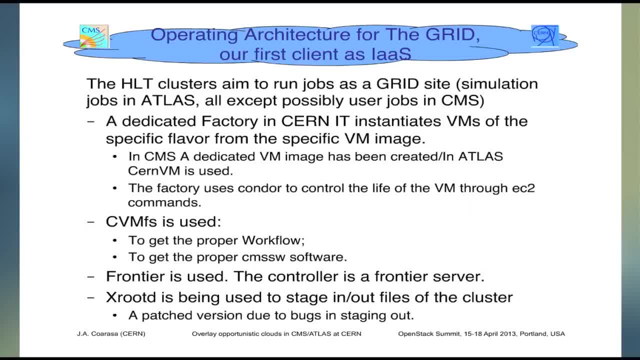 And these services. maybe, if you're interested, I can go into some detail later, But they are very specific to the grid. So these ones here are proxies, kind of proxies for some services that the grid needs And, of course, something or somebody. 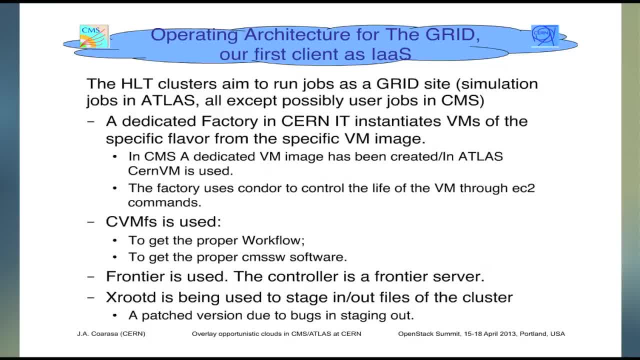 has to control the life of the VMs And this something or somebody is an evolution of Condor, basically. that basically controls. knows how many jobs are there to be done, simulation, reconstruction, et cetera, How many jobs can be sent to all clusters. 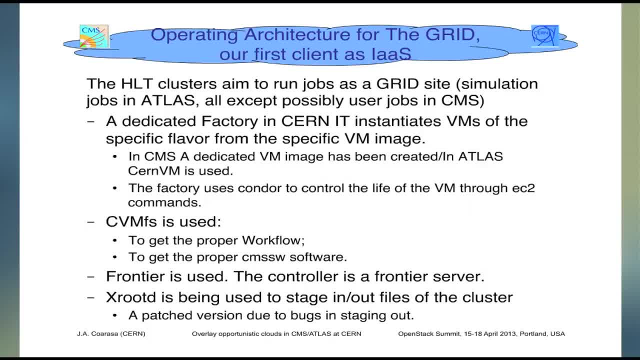 And then he will actually create a VM, instantiate a VM And then the VM will contact back, will retrieve the jobs and will execute them. OK, But this is just the glue to be able to run or grid jobs in clouds. There's a lot of development in this now. 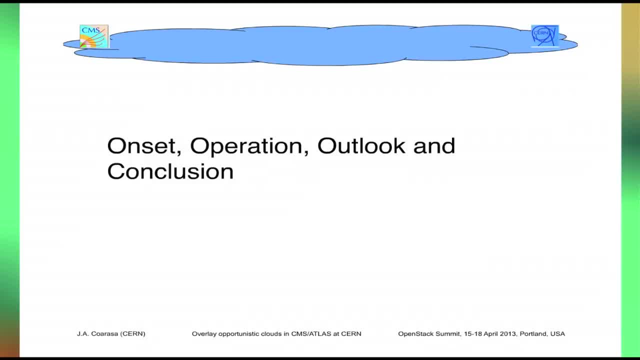 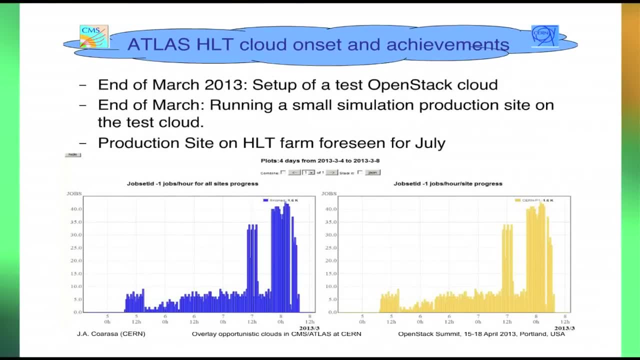 Now let me explain a little bit more the evolution of all of this. This is what Atlas has been doing from, basically, the end of March. There's a typo there. That should be March, beginning of March. OK, So they set up the OpenStack cloud. 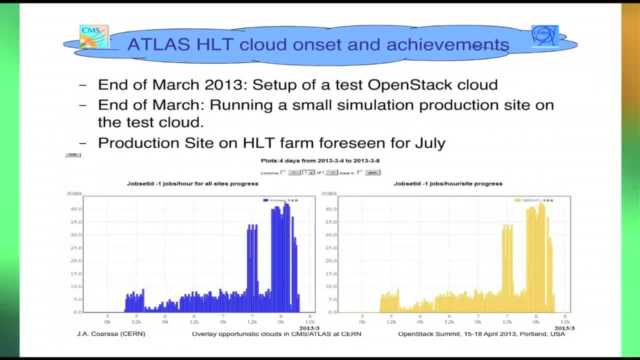 And they were running a small simulation production site on the test cloud. Here you have the results. actually, This is the number of jobs And this is the time So they were able to run in this test cloud that I showed you before. just quite a few jobs. 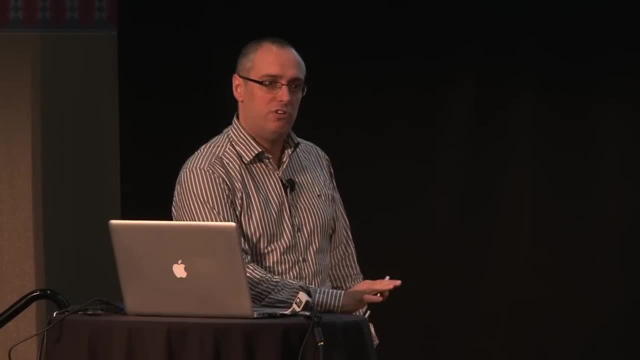 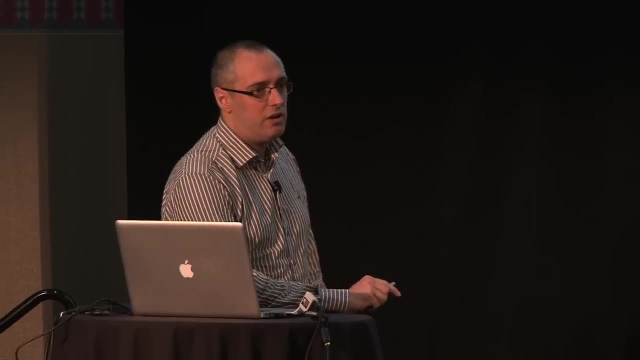 in not a long time, Let's put it this way. But that was just a rack. Now they are deploying it in the whole 1,490 nodes, And they will start running around July. OK, Now what did we do? 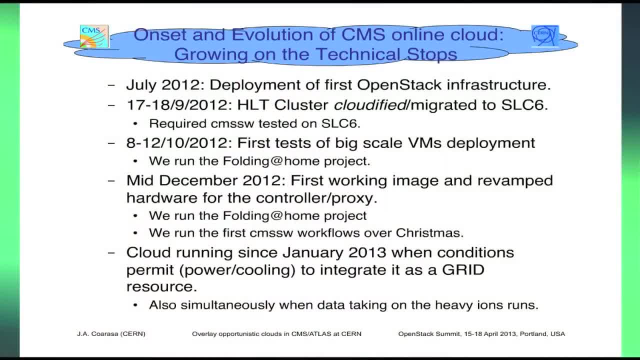 We started back in July But, as I said, we couldn't do much. We could only do one week out of nine or so. So first we set up our OpenStack in a stolen rack, OK. Then after that we were able, after basically a month or so. 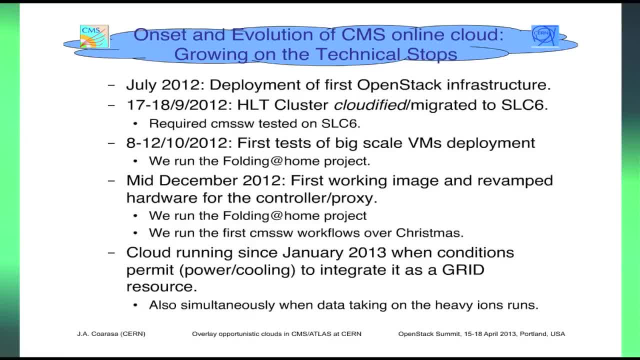 we were able to start well to basically first migrate the whole cluster, because we had to migrate to SLC6 to have proper support for the Nova compute, And then after that we were able to do, in the next technical stop, big scale VM deployment. 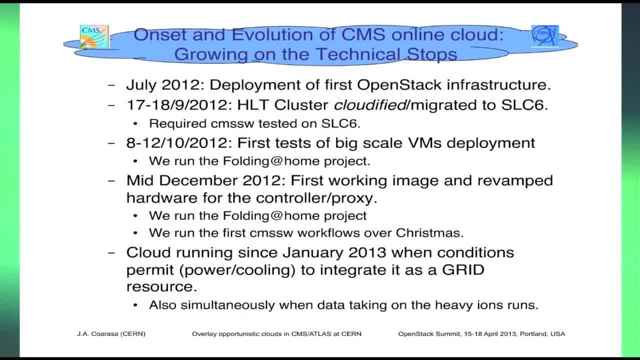 We didn't have our software prepared to do that, or all the other infrastructure around it, So we had to find a way to test it and to see whether it was stable or not, whether we had problems with so many VMs being deployed. 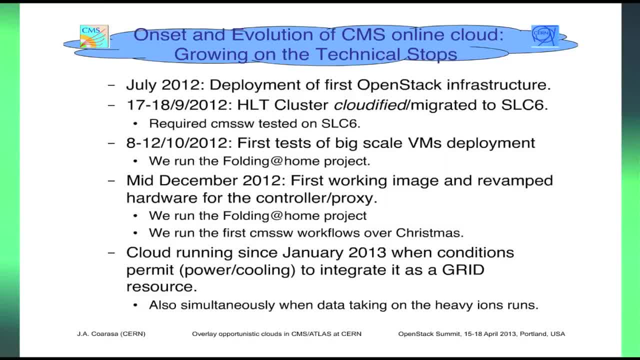 and so on. So Boicek found a project, which is a nice project, which is folding at home. basically uses your CPU to find if some drugs are good to against cancer, Parkinson's, et cetera, et cetera. 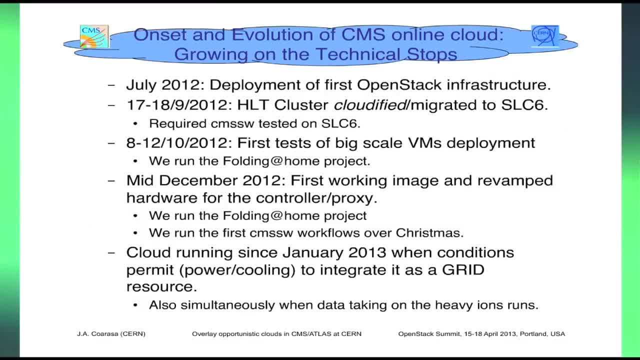 Right. So we ran this project And we were able to run it only like 10 hours before the end of the technical stop Because we had many problems to deploy, et cetera, et cetera. Now, after that, everything went really smooth. 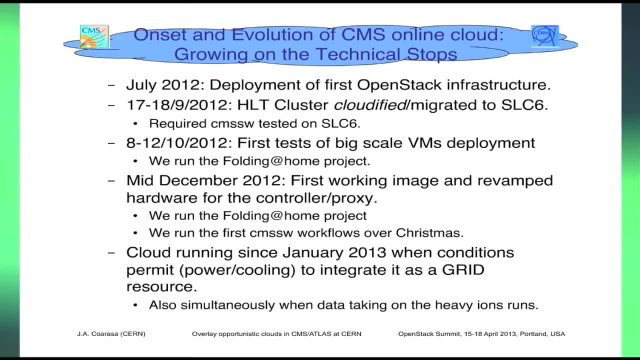 And in Christmas we were able to use the cloud as a cloud for basically three weeks And we ran all software plus the folding at home software, And after that, since January, we've been running the cloud in cloud mode- At least part of it. 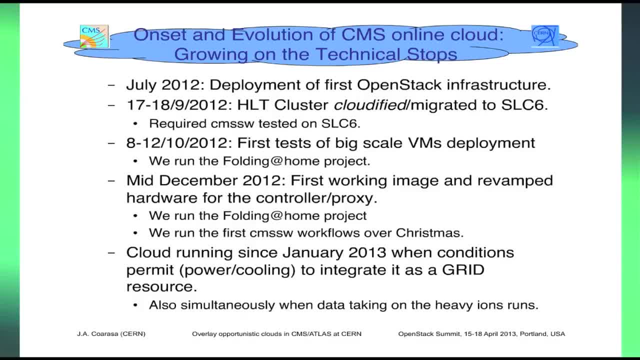 All the time. Now, of course, the whole cluster is being run in cloud mode, Even when we were running taking data for heavy ions, since we didn't need, as I said before, the whole cluster, we just used it. 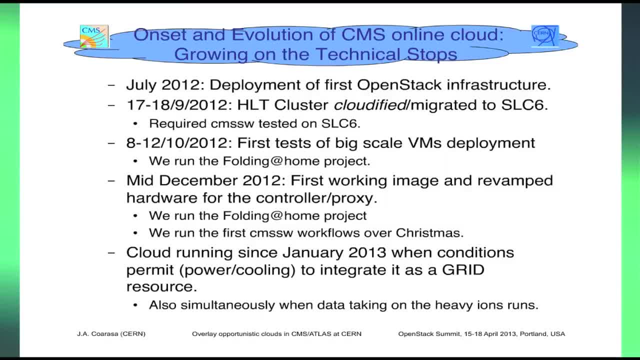 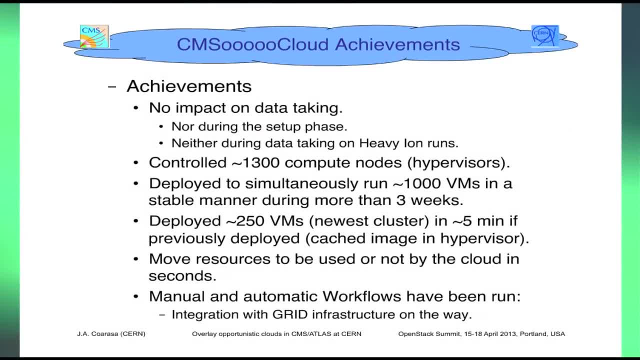 So that was, if you want, the first opportunistic use of the cloud by somebody else, not us. Now, what are our achievements? OK, the first one, which is very important, is no impact on data taking. Nothing happened. 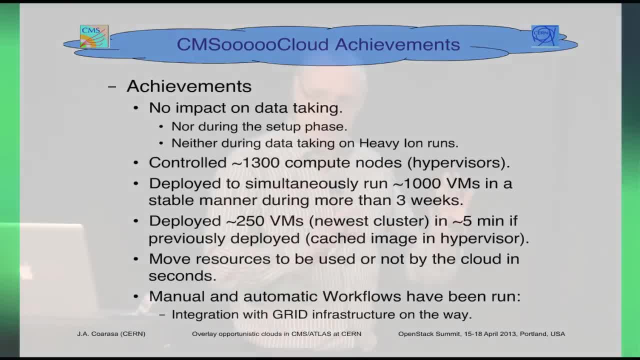 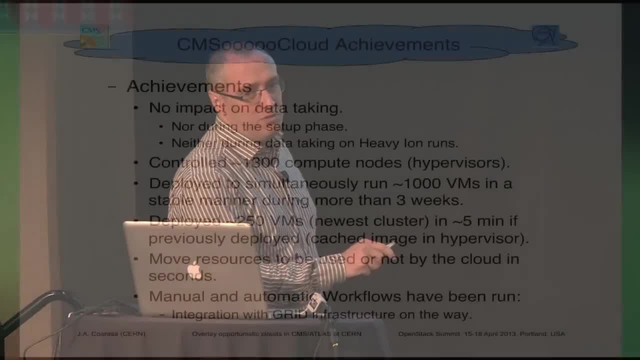 Even if we were actually migrating the whole cluster to have the proper support, et cetera, nothing happened, which was good. Then, when we were taking data, also during heavy ions runs, we had no issue with the data taking either, which was also good. 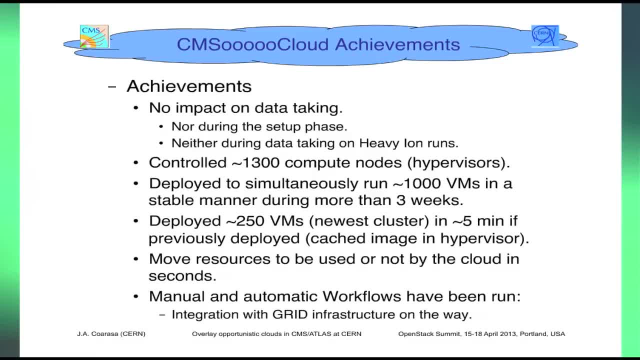 That was the first demonstrator that things could go well. Now we were able to control our 1,300 compute nodes with no problems. We deployed more than 1,000 VMs to run in a stable manner during Christmas More because here I don't have how many of all kinds. 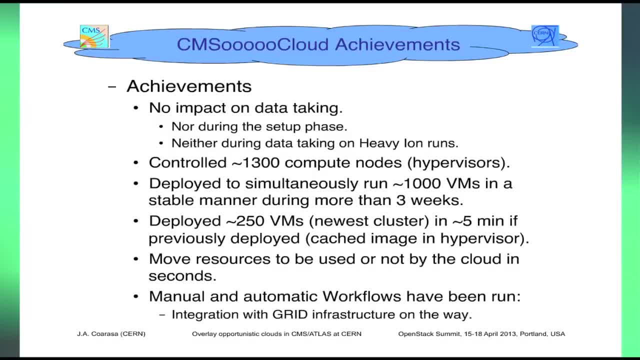 were running. I only know how many of folding at home were running. The other ones I cannot know. And then we are able to deploy 250 VMs in less than five minutes if we already have the image cached. That's important because that's the part that we think that we 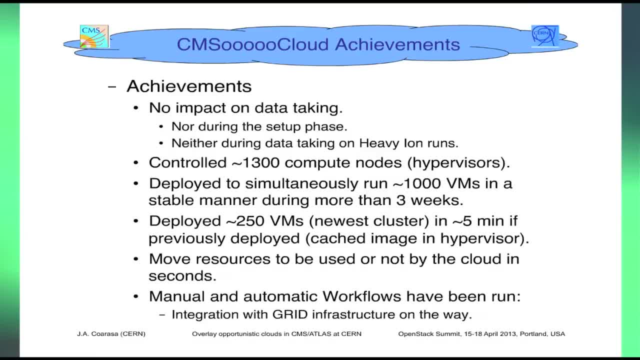 are going to be dedicating more often to cloud computing. These are the faster computers and this is the part that for us is important. For example, we used when we were taking heavy ions data. Now we can move resources to be used or not. 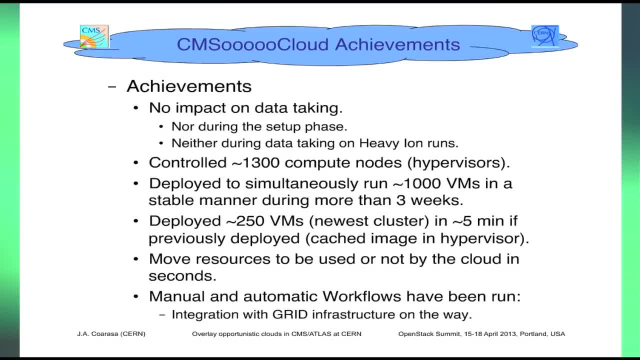 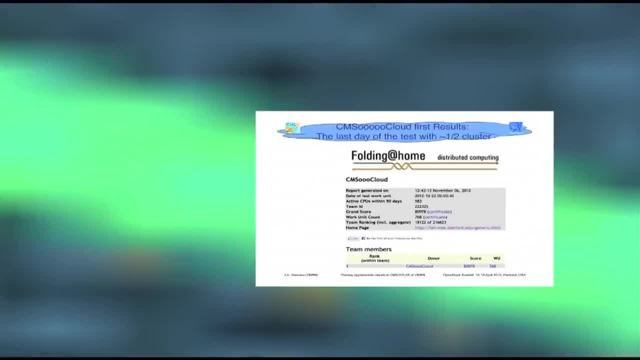 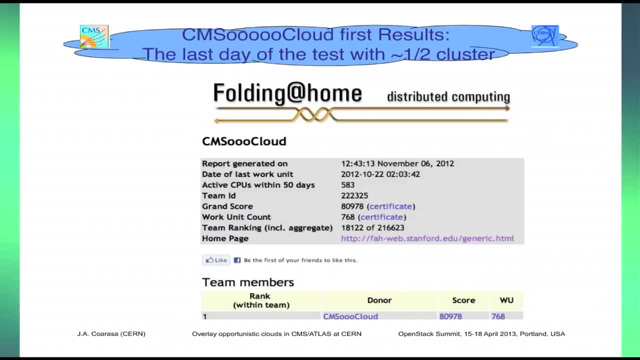 by the cloud in seconds And we've been able to run automatic and manual workflows of all software inside the cloud. So this is the certificate that we were able to accomplish some work units after only eight hours of running our cloud, The first time we tried. 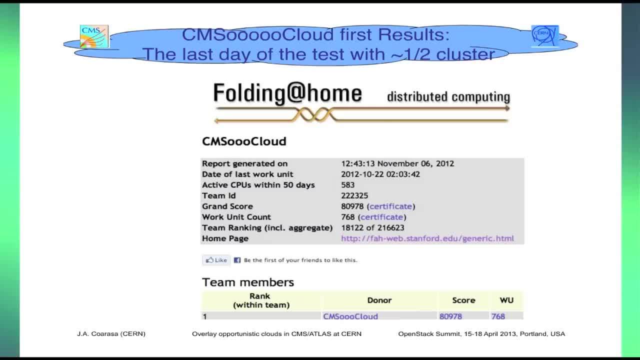 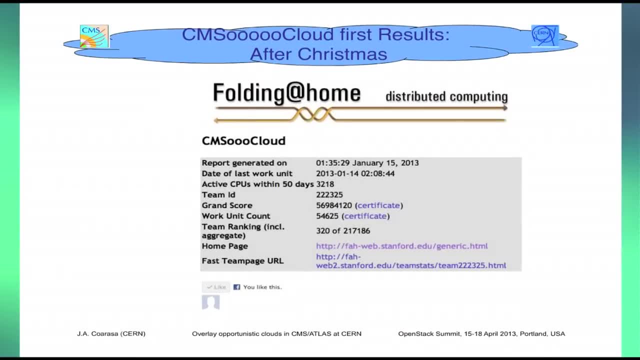 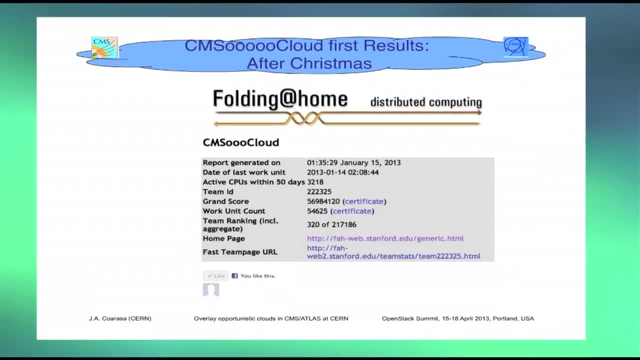 And we were not OK. we were basically 18,000. And after Christmas, something happened. Three weeks running, we went up to 320.. We had been able to do 54,000 work units. And, of course, we can also do our job, which is our jobs. 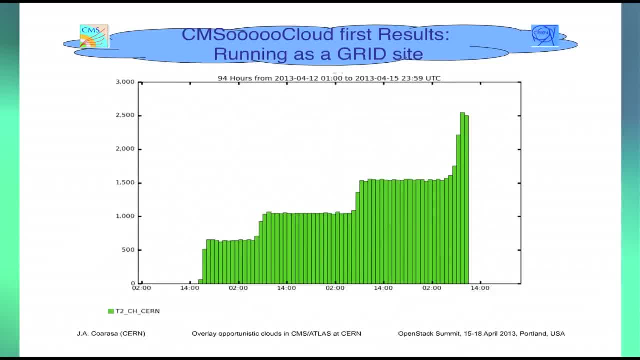 This is number of jobs and this is a ramp up that they tried only a few days ago, And you see that we can run in only a couple of hours, a few hours, up to 2,500.. And here we are only using. now we are only using. 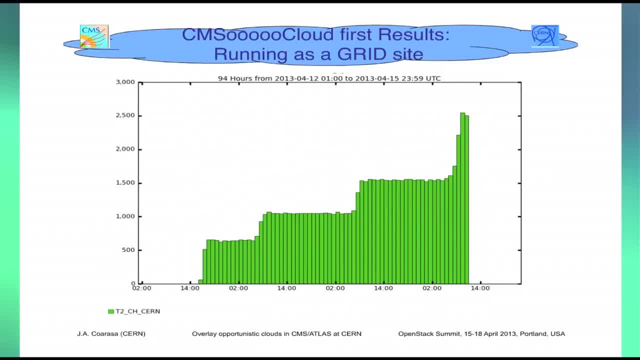 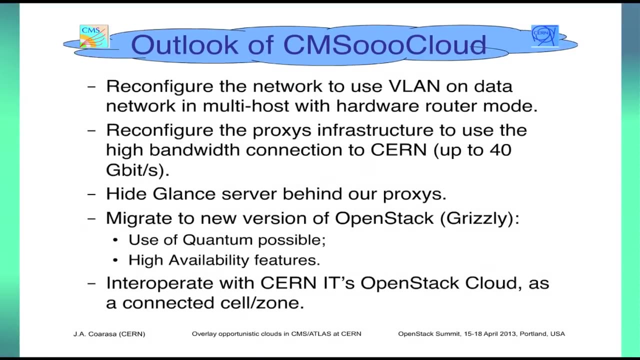 I think it's 40 hypervisors, because we don't have power now to run, But this was only because we had a power cut last week. OK, So now what is the outlook for us? We now will reconfigure our network. 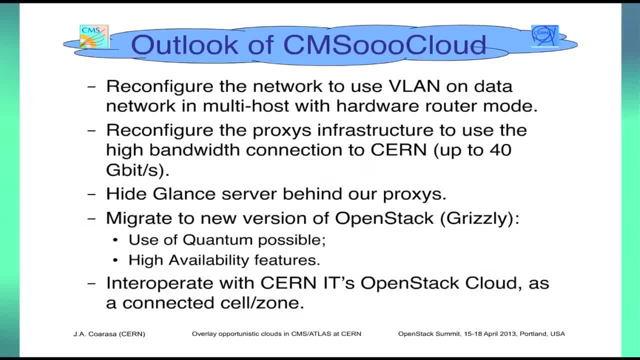 Now we can, because basically we are not running And we will add VLAN. We will run in multi-host and with a hardware router, probably. So we will probably still use Nova Network. That's not clear. We may use Quantum. 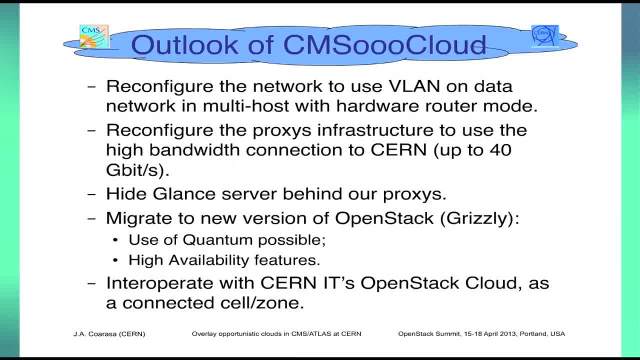 We will reconfigure our proxies infrastructure to use the 40 gigabit link that we didn't use so far And we will hide glance behind our proxies So that actually the distribution of the image is not taking forever when we distribute a new image. 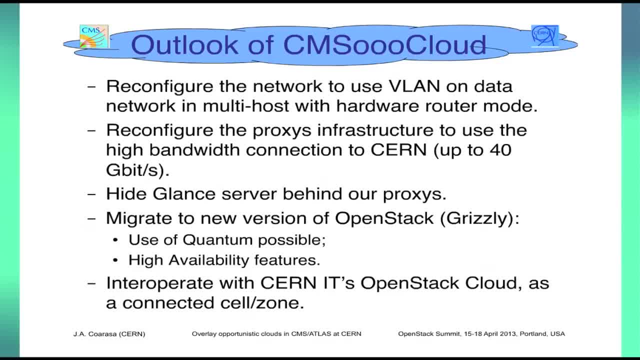 And we will migrate to Grizzly. I've been hearing many HA high availability sessions here And we will definitely go to high availability Now that the proof of concept phase is finished. we really think that we have to go this way And maybe in the future we can just 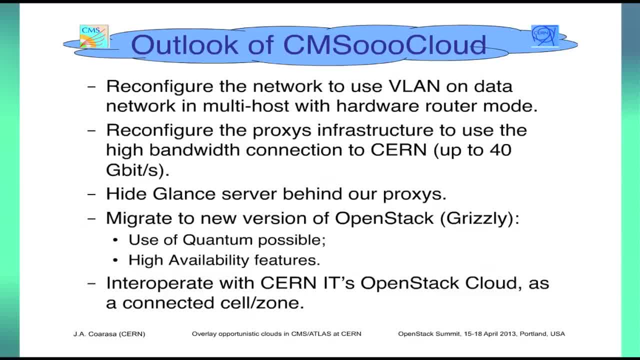 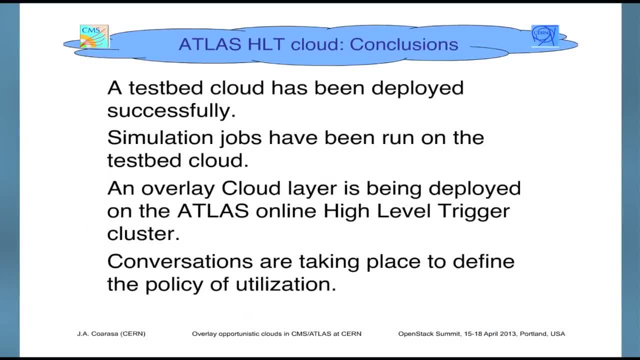 interoperate as a network, As a connected cell or zone or region to the CERN cloud, because now we are separated clouds. Atlas has been able to deploy it successfully, the testbed cloud also to run simulation jobs on the testbed cloud. 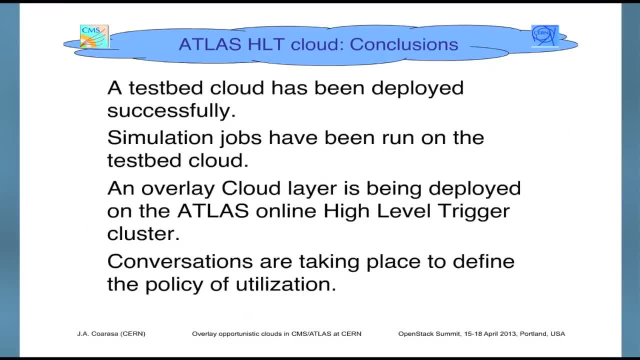 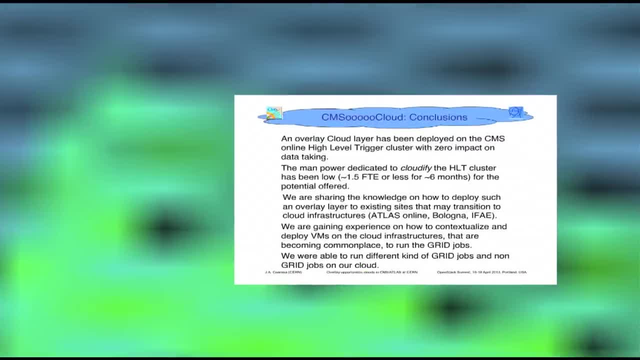 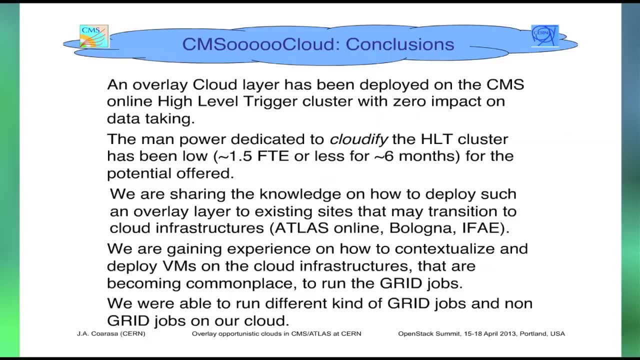 Now they are actually deploying the cloud on the high level trigger cluster And they are defining how they will be using their cloud. As I said, we've been deploying the CMS online high level trigger with zero impact to data taking. We have not been dedicating a lot of manpower data. 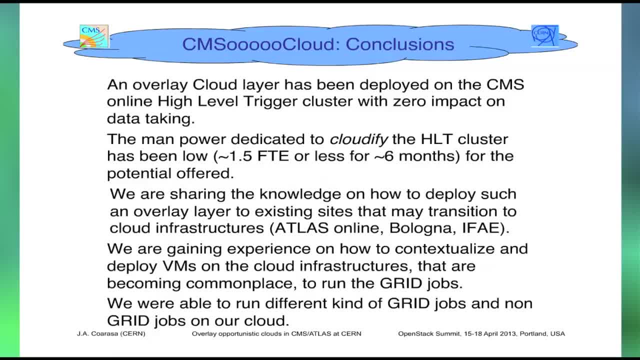 It's been like 1.5 FTEs for a few months, where a few is six more or less. We are sharing our knowledge now with other groups. Actually, we shared it with Atlas. They decided that it was worth to go more or less. 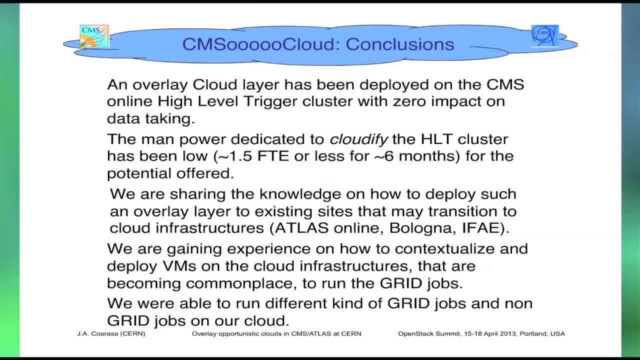 the same path We've been sharing with other groups that basically are grid groups that are migrating to clouds, And in this sharing we also share another thing which is a little bit more specific to us. It is the way in which you can run grid jobs on the cloud. 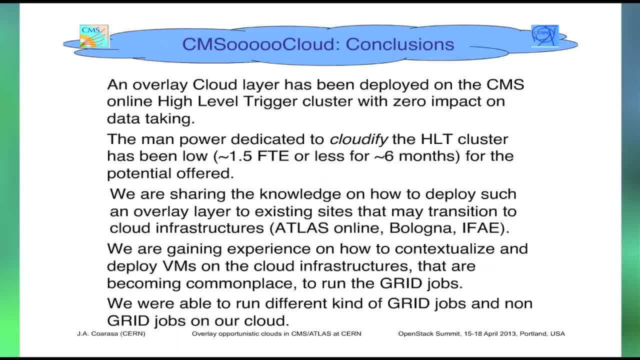 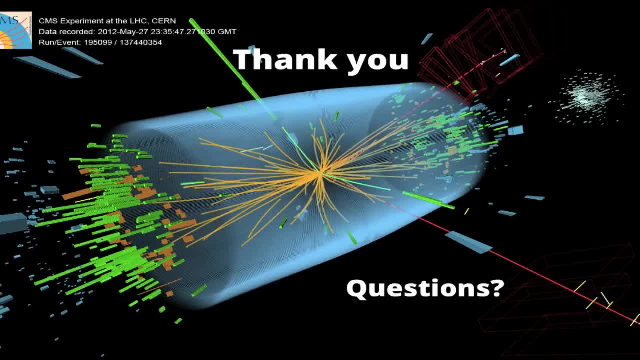 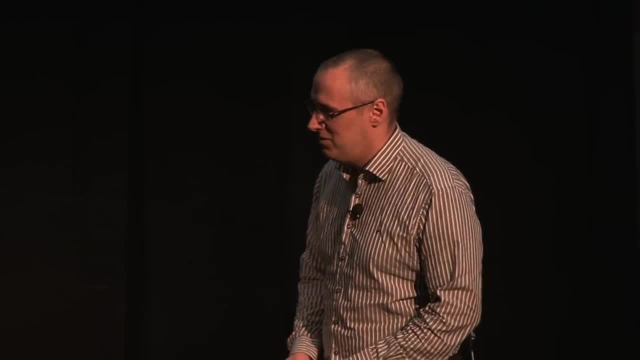 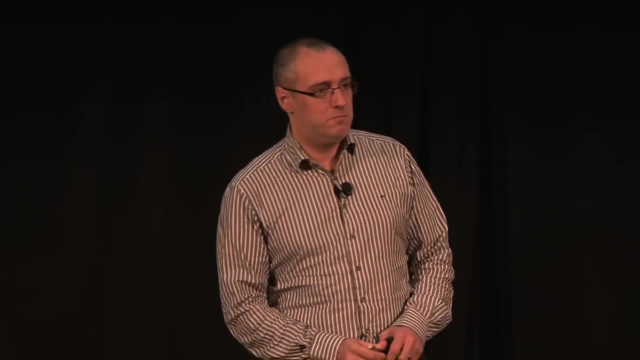 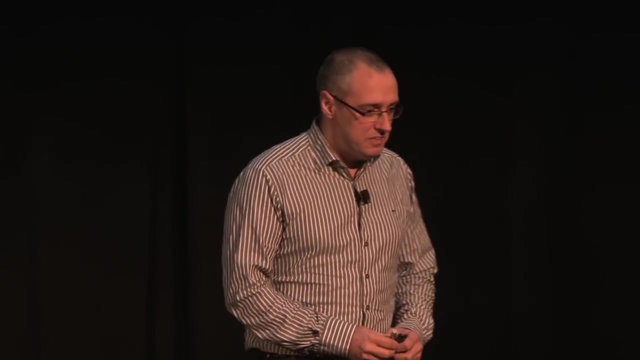 And, of course, we've been able to run these jobs in our cloud. Now, I think I was not boring you very much, Thank you, And if you have questions, The question was: are you using Swift for storing data? And the answer is no, because we are a little bit different. 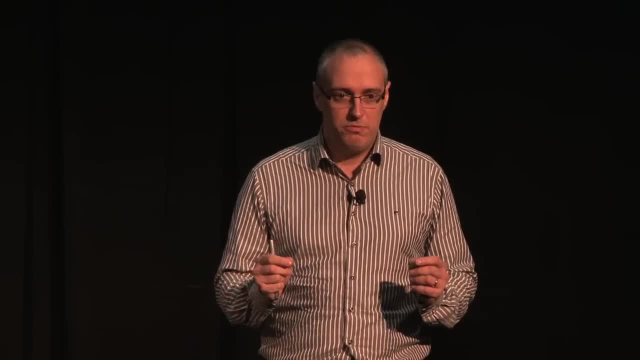 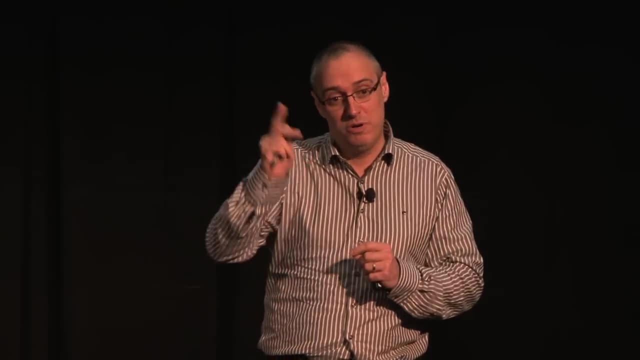 in this meaning we run jobs. These jobs basically analyze data. The data is somewhere else, So if we lose it, we don't care. If you lose the job, you also don't care, because you will repeat the job somewhere else. 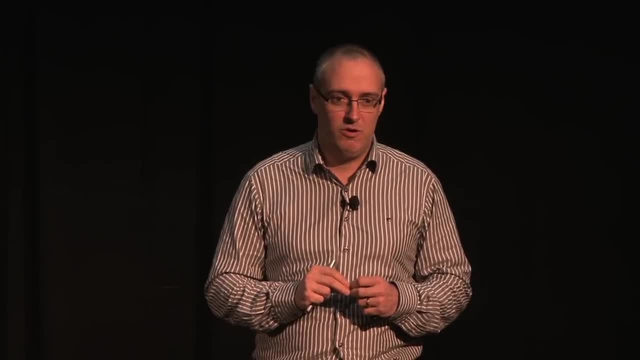 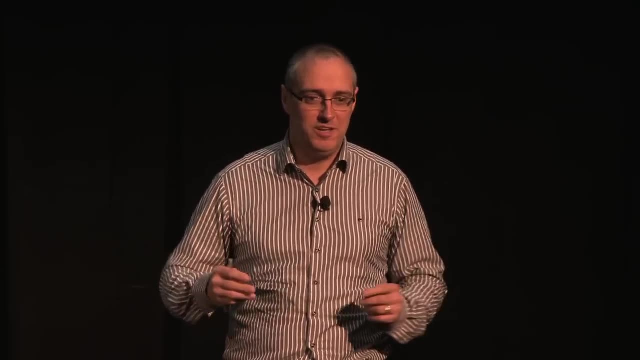 So in reality we don't have a backend of persisting storage or anything. Basically, we use the local disk And if they fail they fail, They will go somewhere else. We are thinking, maybe, that if we want to do some other things on top of this, 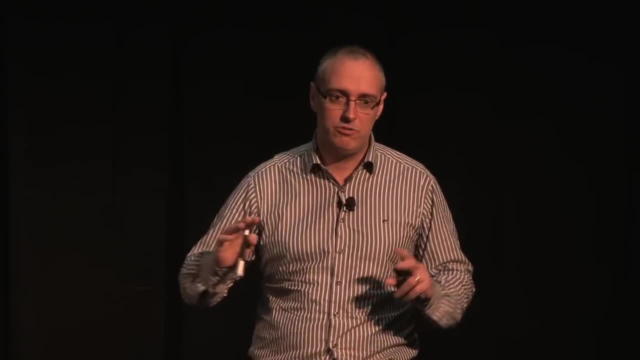 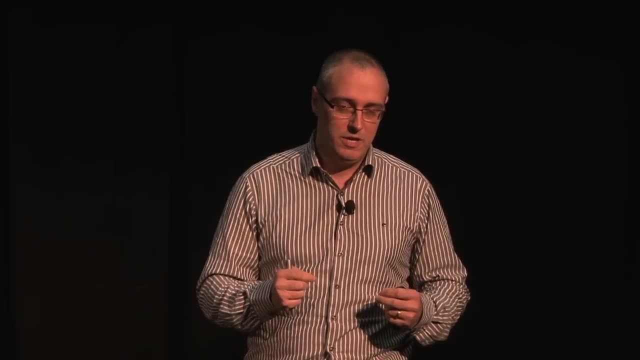 we will use the cloud Because so far we use the cloud only for this. We also have our virtualized services that we use other means to basically use them. If we go and integrate our virtualized service inside the cloud, then we will need it. 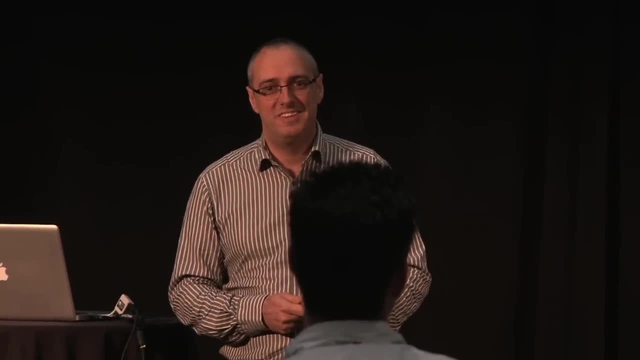 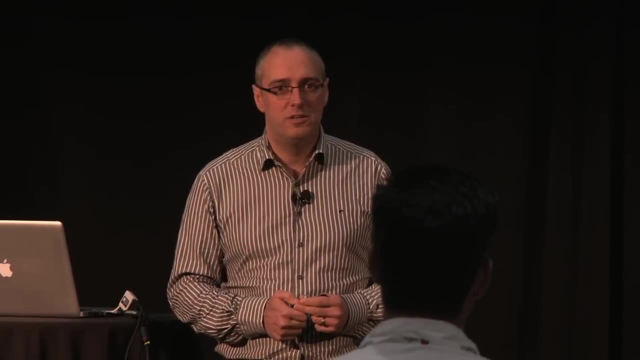 I'll just stand up and ask. So I've been a little bit out of. I used to work for Slack, so I know a little bit how the data moves, So we used to just drop data onto AFS and magically show up someplace else. 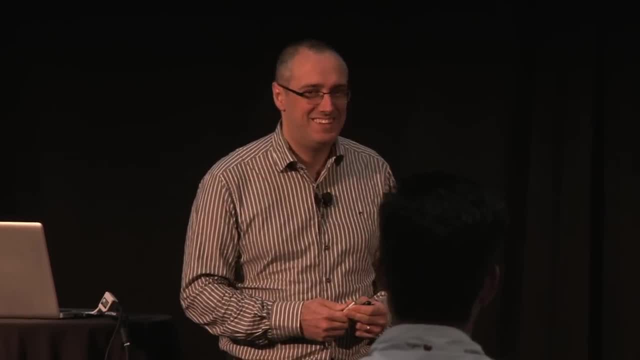 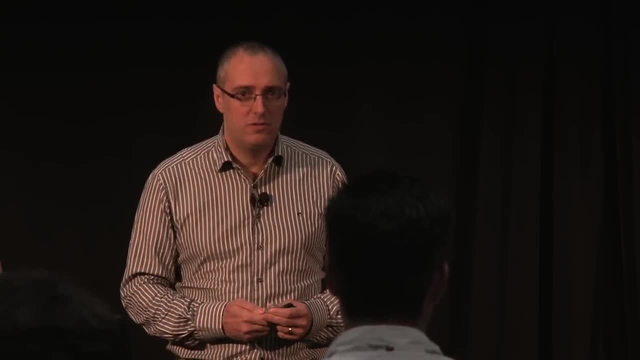 and drive everyone crazy across the world as the data moved trudged across. We generally pull data off of HPSS pretty manually as well and drop it on AFS. Are you guys still kind of doing that manual process And have you been thinking about some way? 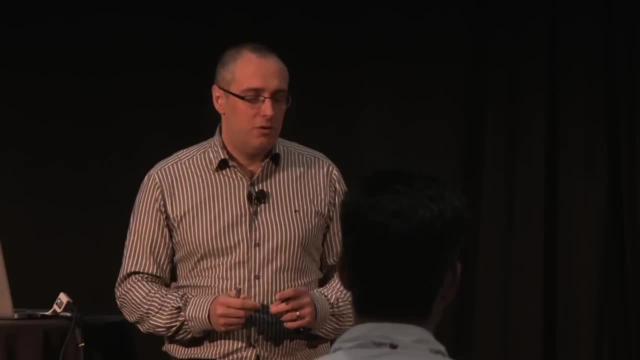 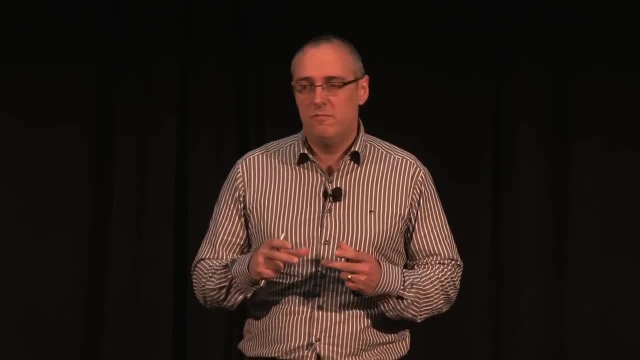 of automating some of that? if you're not, Do you mean OK, All the data that is generated in our data acquisition system? all of it happens automatically. I mean the transfer to tier 0,, tier 1,, tier 2,, et cetera. 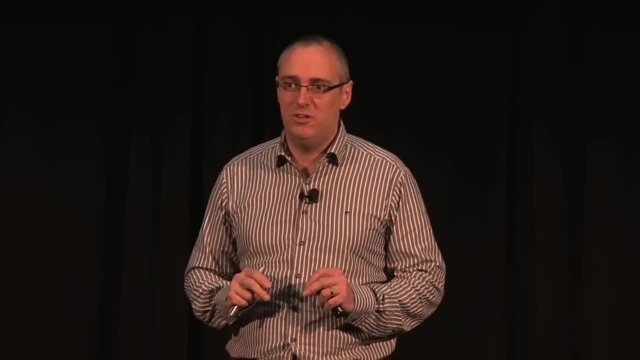 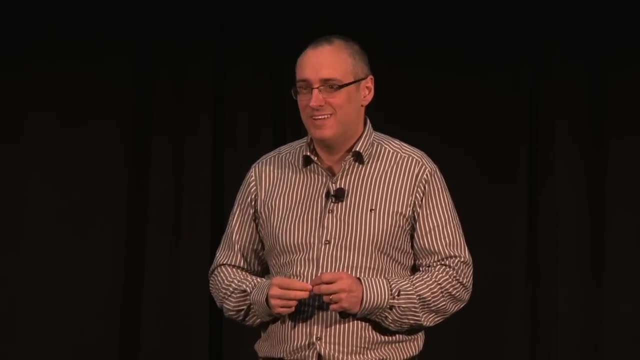 is completely automatic And it uses some in-house developments, But it's not through AFS any longer. no, The big data, no, I mean the local holdings, The homes of the users. they are still in AFS most of it. 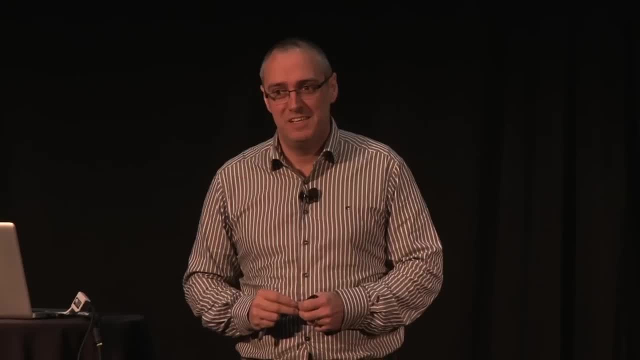 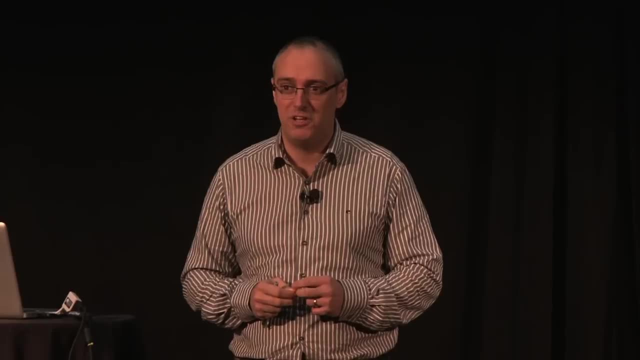 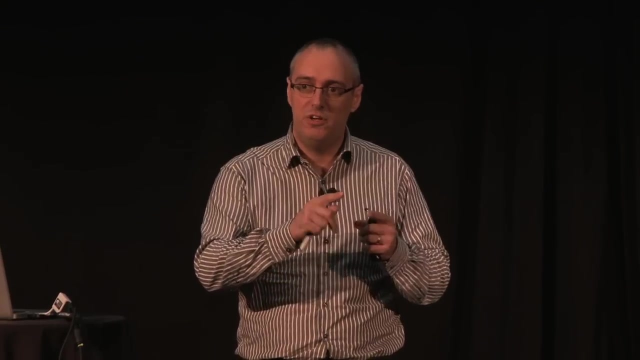 And you can have it if you want, But no, Not this big chunk of data. There is some in-house developments called FedEx, et cetera, et cetera, that use basically to transfer in an automatic way. The data is taken and it's certified that tier 0. 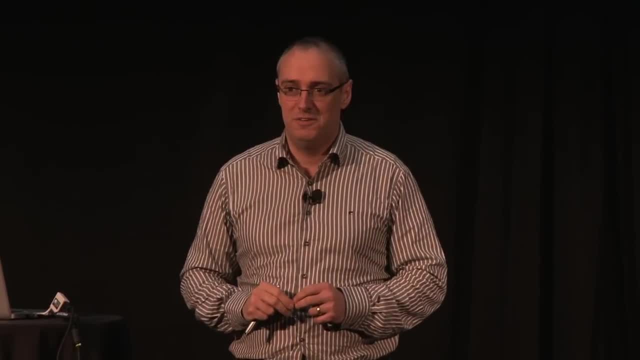 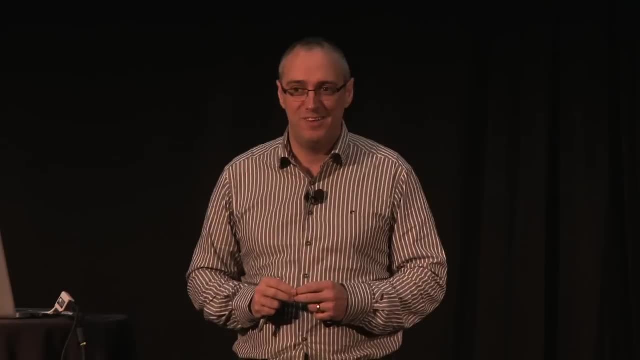 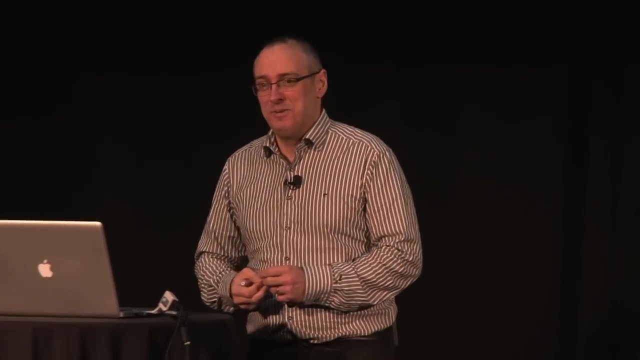 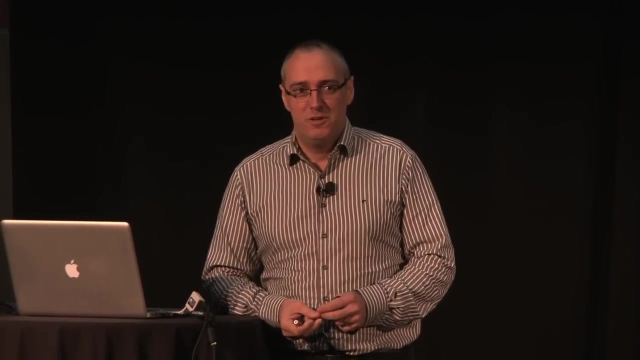 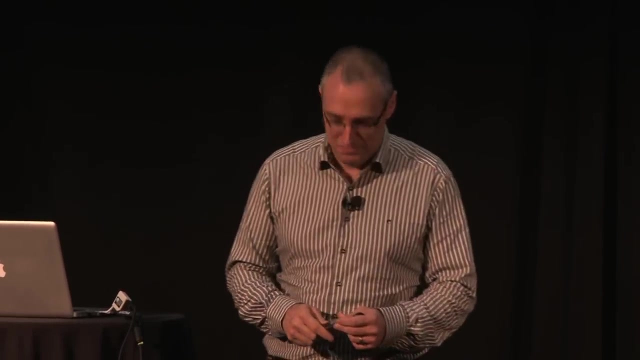 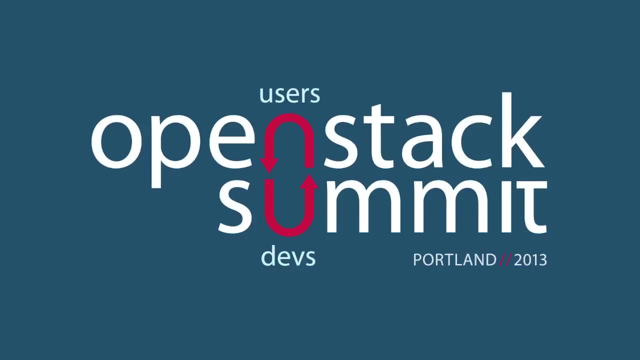 goes to tier 1. And this is completely automatic. I'm not an expert. I'm not an expert in that. I cannot tell you exactly. Maybe Tim knows. OK, There is no more questions. OK, Thank you again, ANDREW PETTERS.